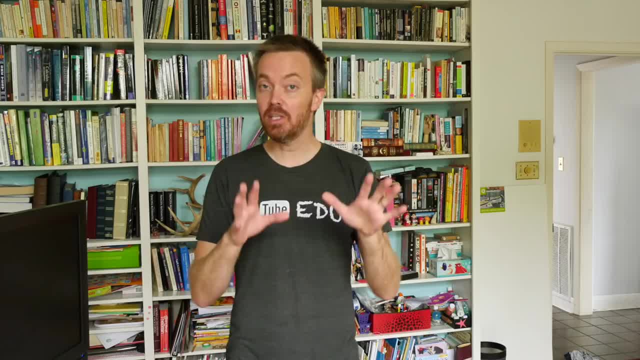 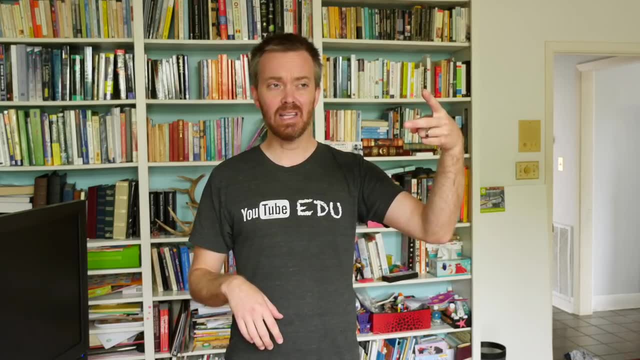 that, even though those two numbers are public, the only person that can decrypt those messages are the intended recipient. And you might think: well, geez, you know, those two numbers are public and that's what it hinges on. Isn't it possible to use those to to sort of hack into those numbers and figure out what? 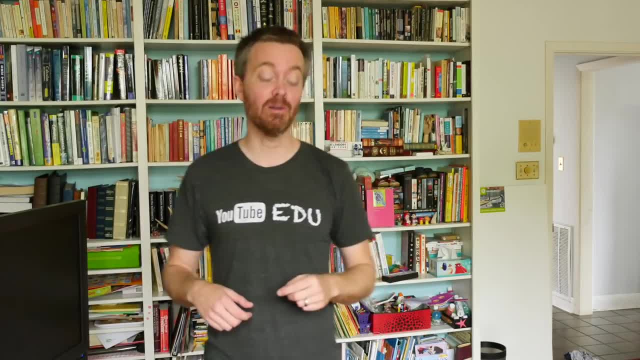 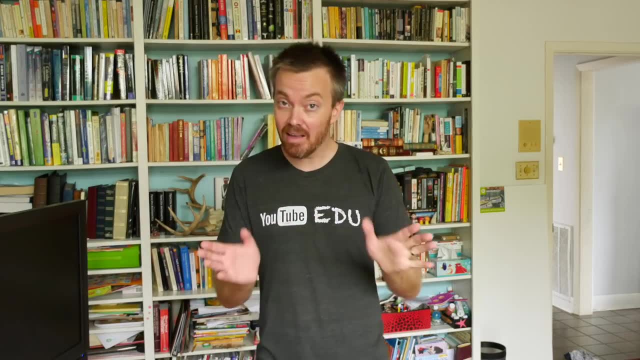 the message says: And again, that's the magic, That's the really cool part. It turns out. you know the, the numbers that are public, the one that's going to be really important. it's going to be a large number. So in my upcoming demonstration, I'm going to show you how it actually works. 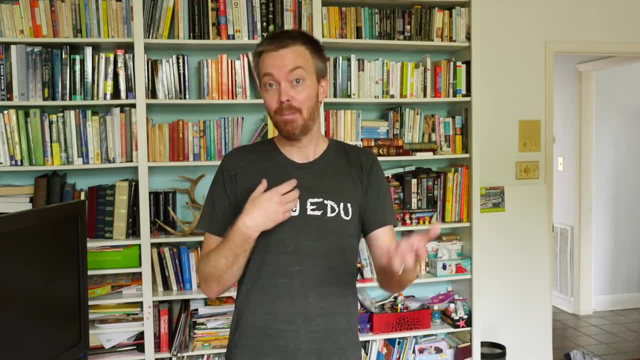 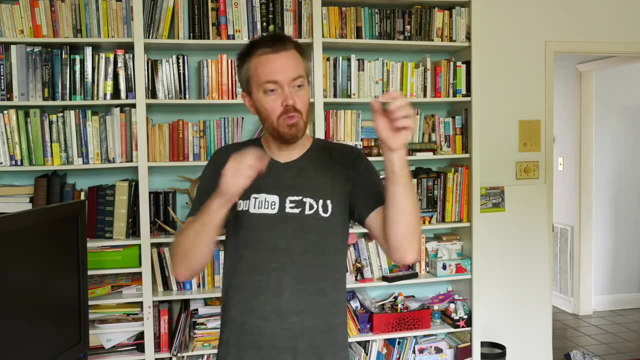 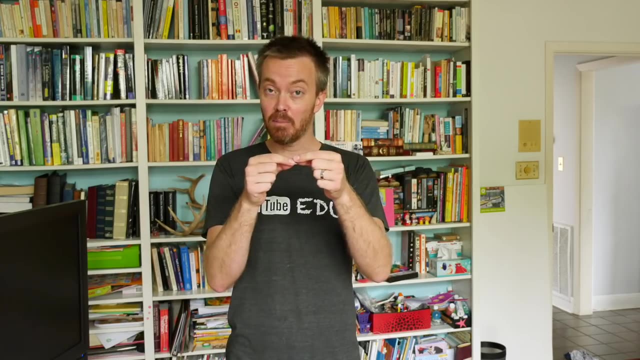 I'm going to pick some small numbers just to make the mathematics a little more manageable. In reality, we use gargantuan numbers and this is the point, These numbers, one of the numbers you use. the fact that it's useful is you take two prime numbers and multiply them together to get that number And to be 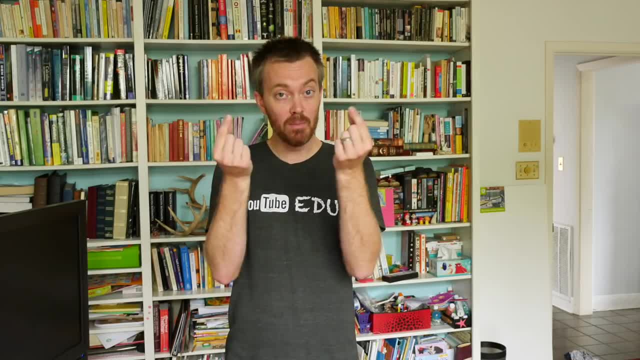 able to decrypt the message, you need to know what two numbers it came from. So you might think, well, geez, I've got two numbers and I need to know what two numbers it came from. So you might think, well, geez, I've got two numbers and I need to know what two numbers it came from. So you might think, well, geez, I've got. 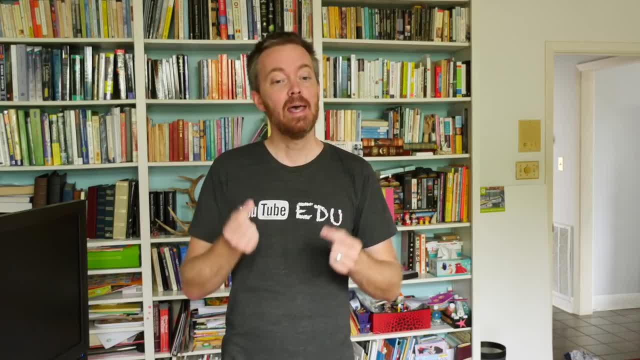 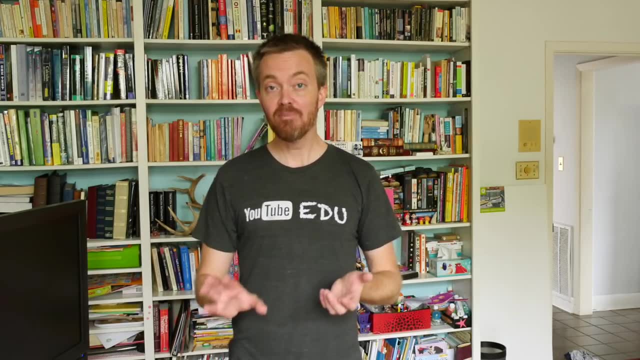 this number. certainly, I can factor it and find those two factors, But this is the problem, and this has been something that's been open for thousands of years. It turns out that factoring is actually a really hard problem. A lot of mathematicians are of the opinion that it's going to be, it's just something. 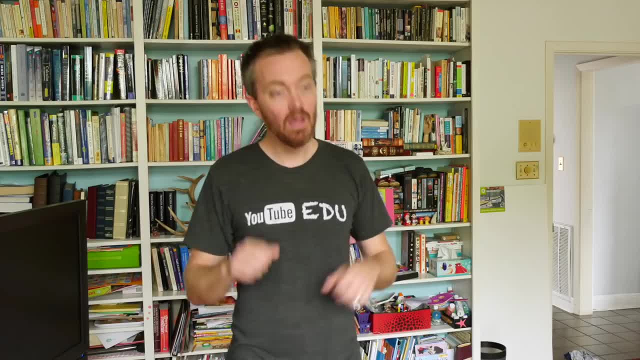 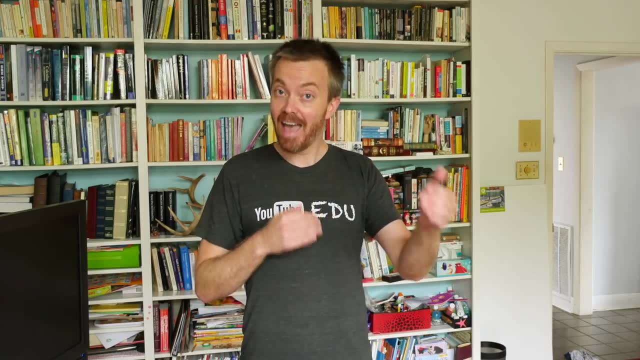 that there's not a good solution to it. Well, it turns out there's actually something known as Shor's algorithm. But Shor's algorithm? it provides a fast way of factoring, But the problem is- and this is the catch- you need what's known as a. 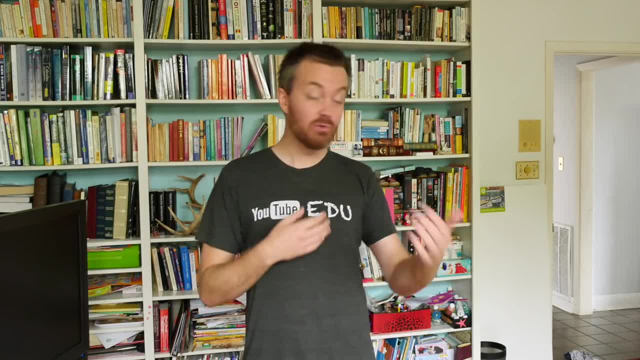 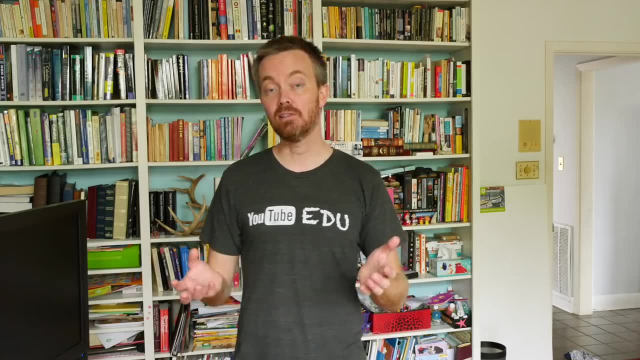 quantum computer. We don't have quantum computers yet. I was reading something the other day. I think we're getting close to maybe having something viable, And if quantum computers do come into existence, this current form of encryption will no longer work. So you may think: oh no, what's happened? Fortunately, people are 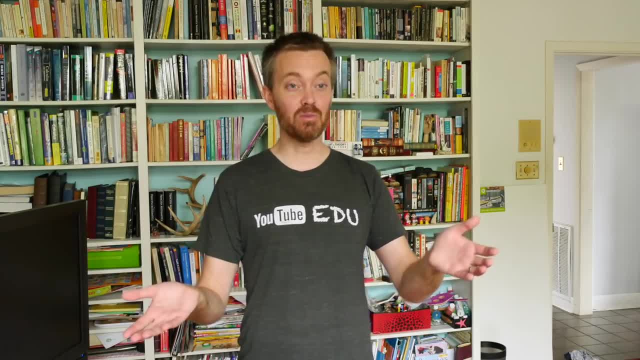 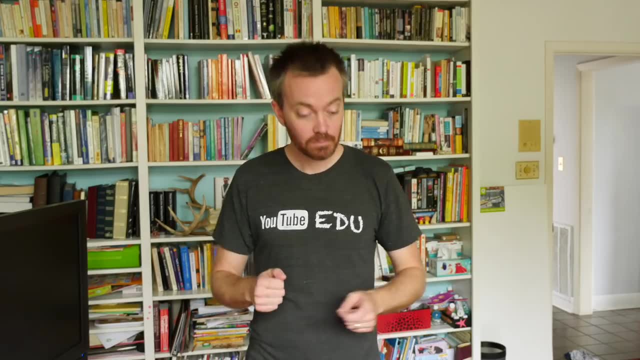 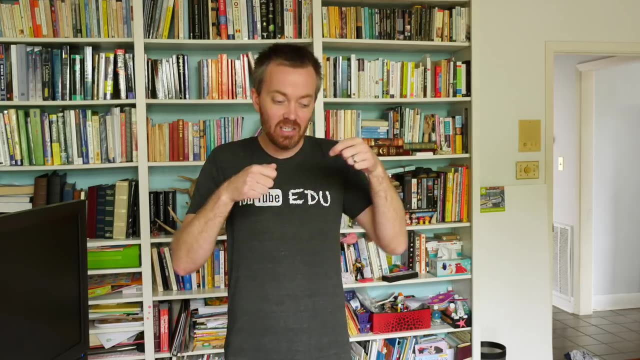 already working on algorithms, post quantum algorithms. So even if quantum computers do come into effect, there's there's a backup contingency plan for encryption. So okay, so you can't factor these numbers And again, that's the magic. But to actually encode a message, that was the difficult part. So 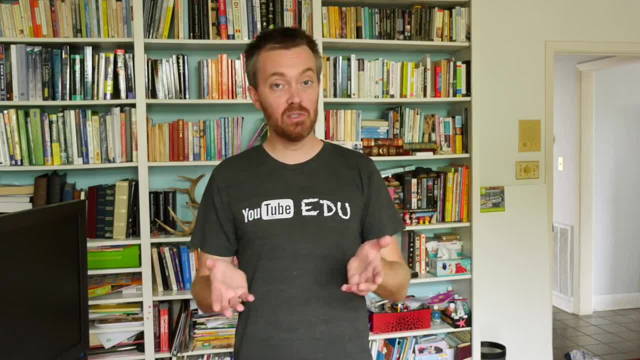 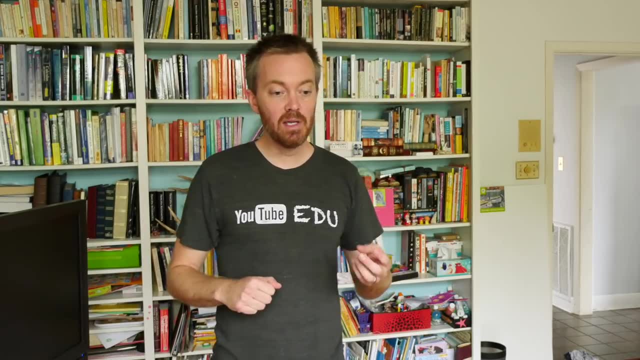 mathematically, they had to come up with a function And we now call these one-way functions. And so if you want to think about, you know, an example of a two-way function. a two-way function would be something like doubling a number, right? 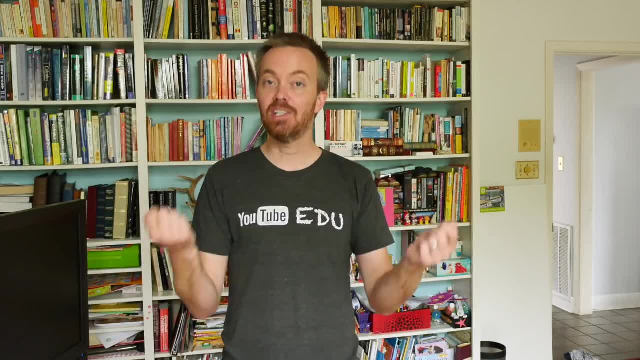 That's easy to undo. So the idea of a two-way function is it's easy to undo, right? So if I double a number, hey, I divide it by two. I'm back where I started, No problem. That's a simple example. 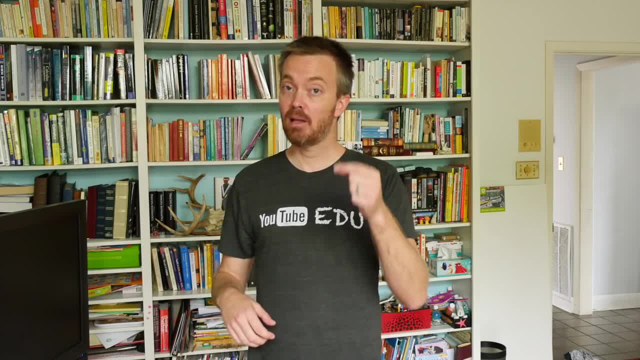 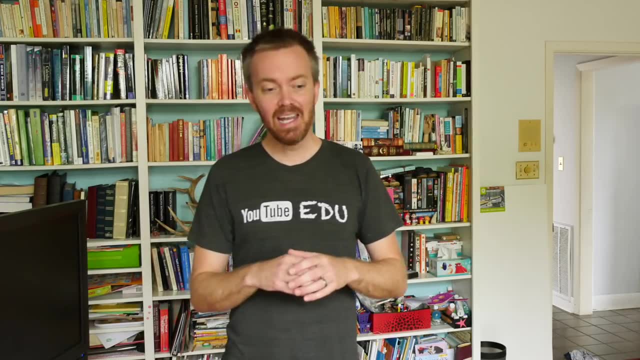 The one-way function we're going to use is based on modular arithmetic And I'm going to briefly talk about modular arithmetic in my demonstration. And again, you know it might be new for some of you. It's nothing super complicated And we'll do a couple quick examples just so you can get a feel of 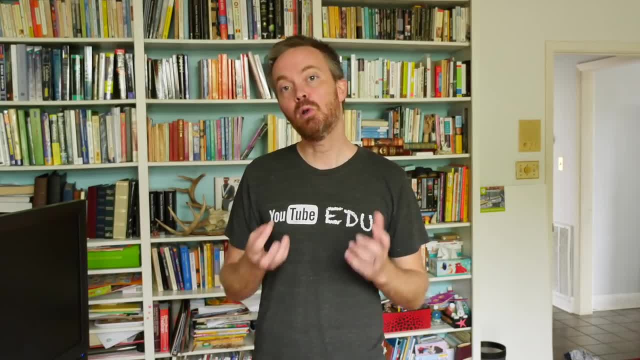 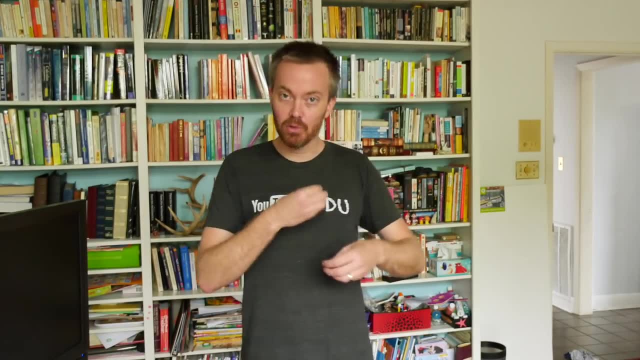 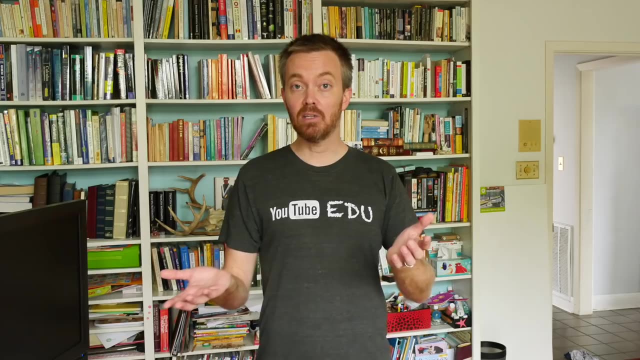 it. So mathematicians tried to find this good one-way function for a long time And everything they found- it was always basically possible to work backwards and figure out what the original message was. But eventually people came up with this idea of using modular arithmetic to come up. 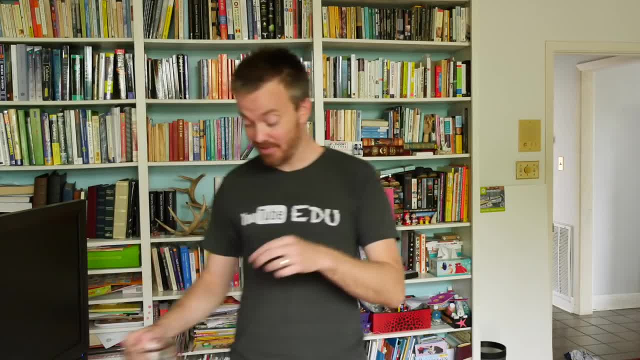 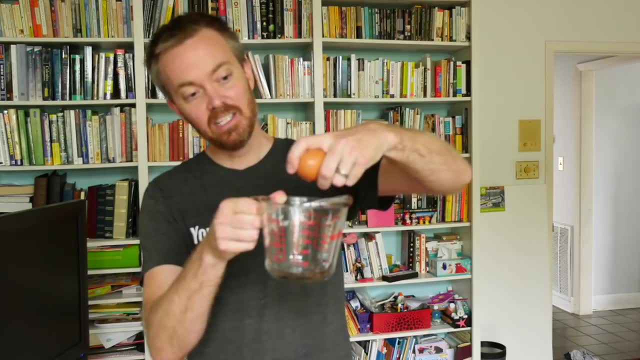 with a good one-way function And in real life, a simple one-way function, just to give you an example, is that of cracking an egg, right? If I take an egg, I like to cook, so I'm going to use this egg later. That's a simple example of a one-way function, right? 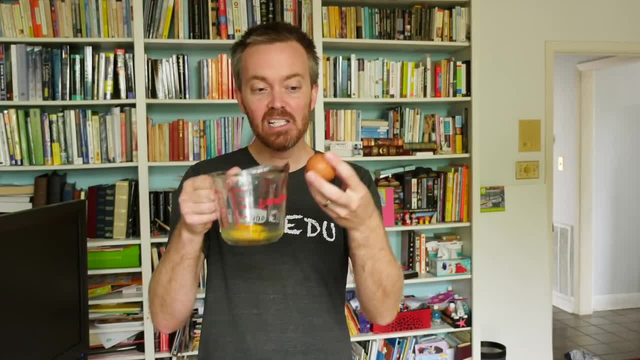 Because it's easy to crack. but it's impossible to now take this egg and restore it back to its previous state. 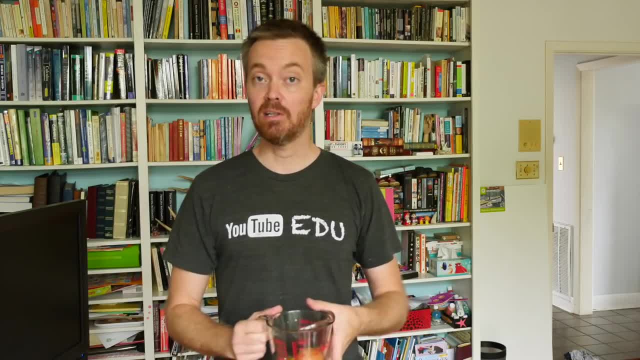 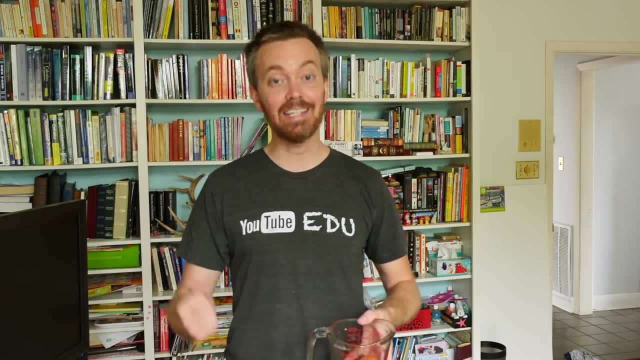 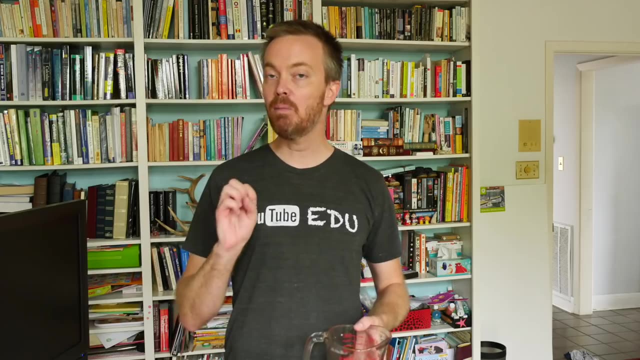 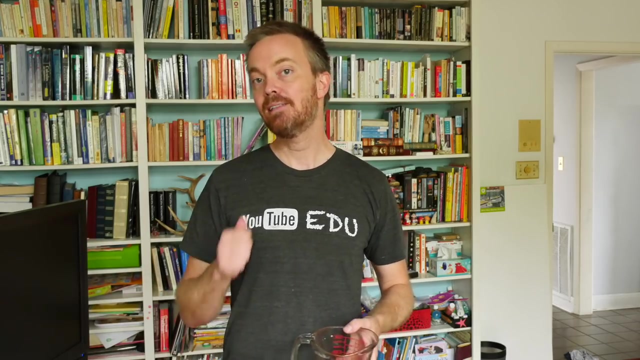 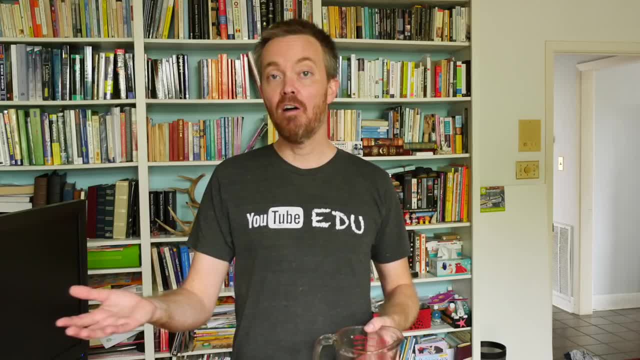 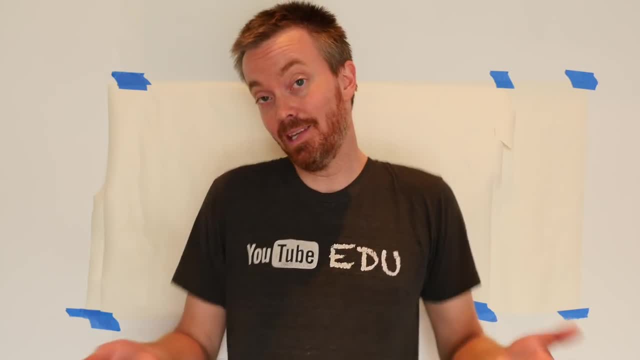 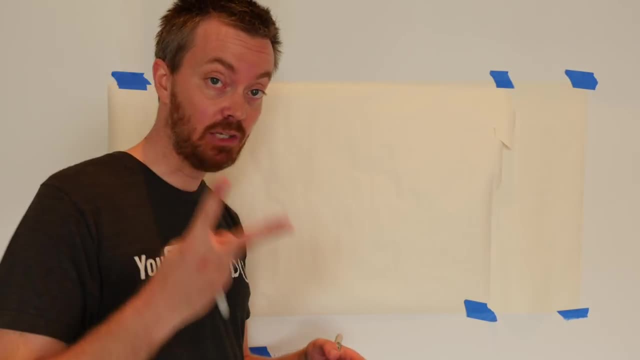 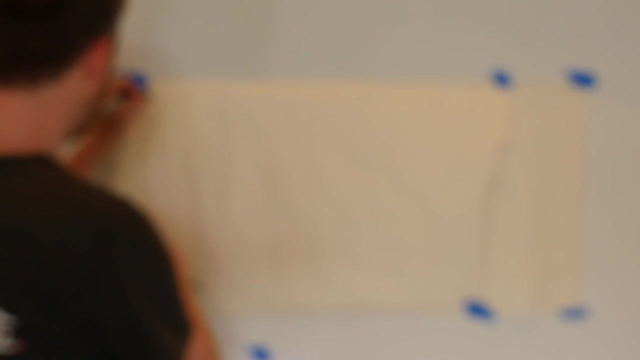 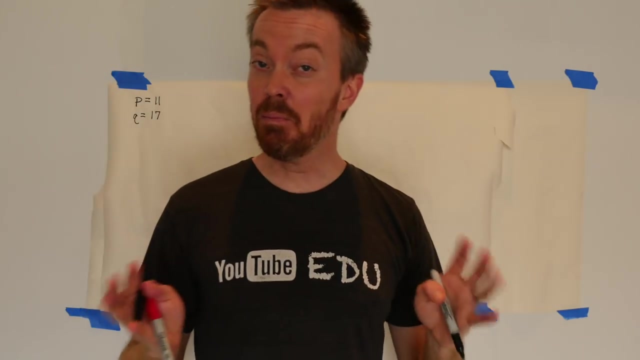 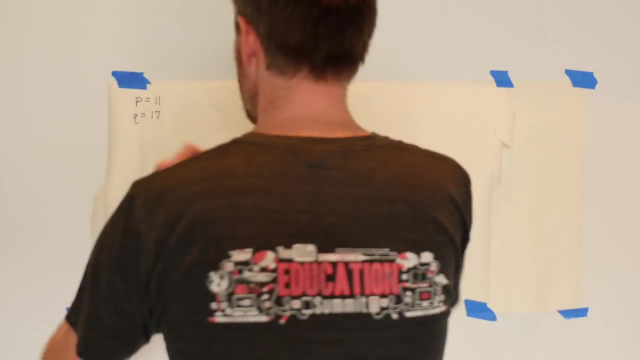 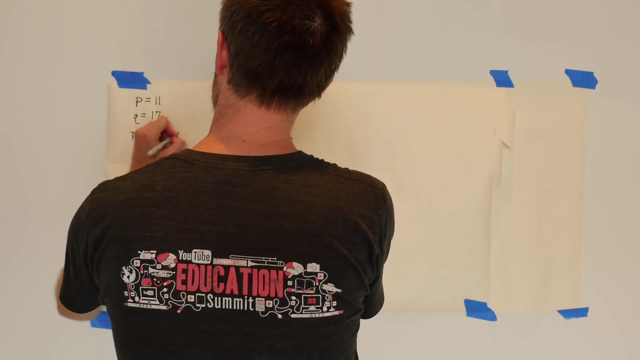 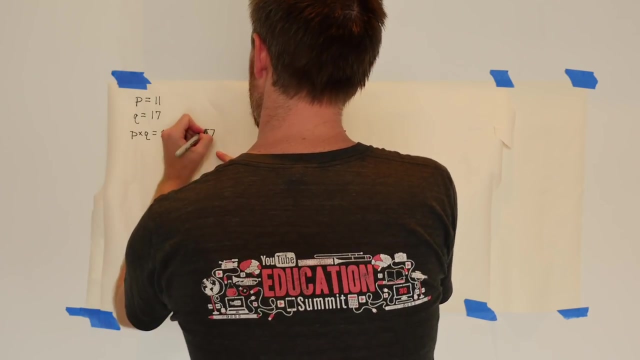 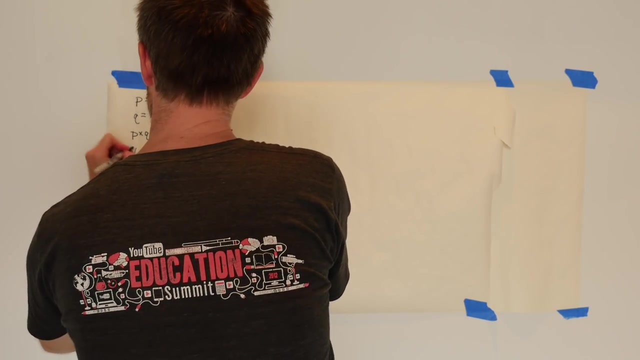 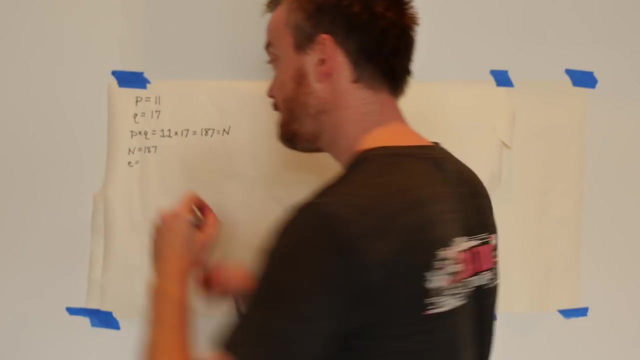 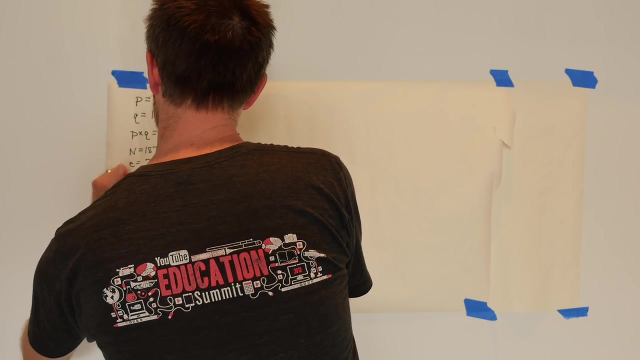 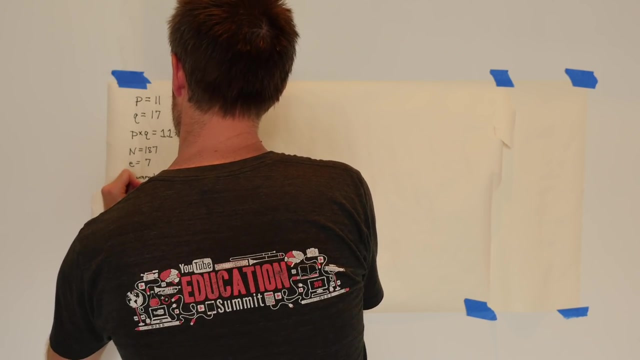 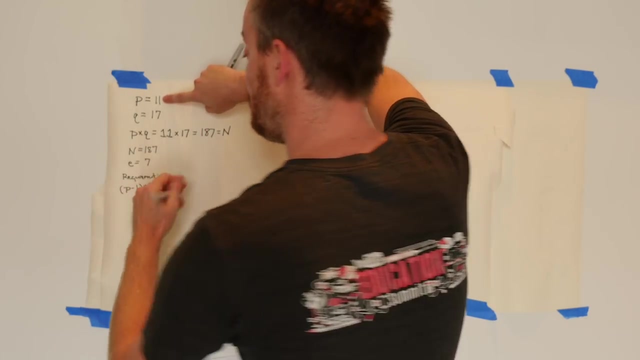 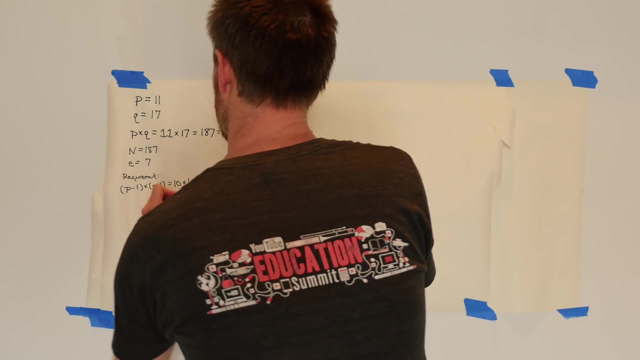 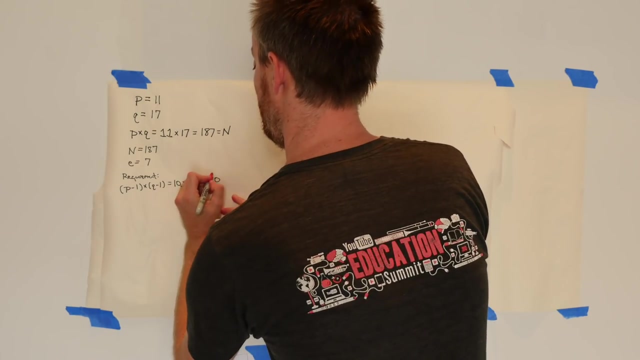 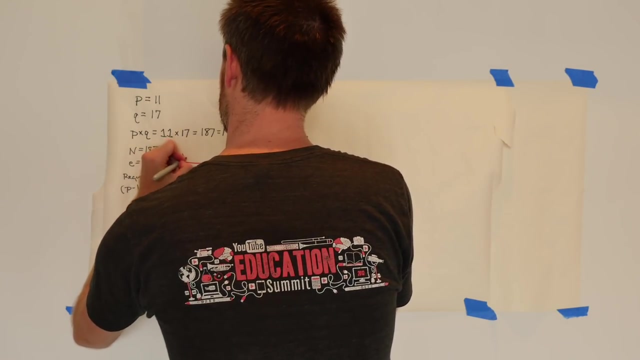 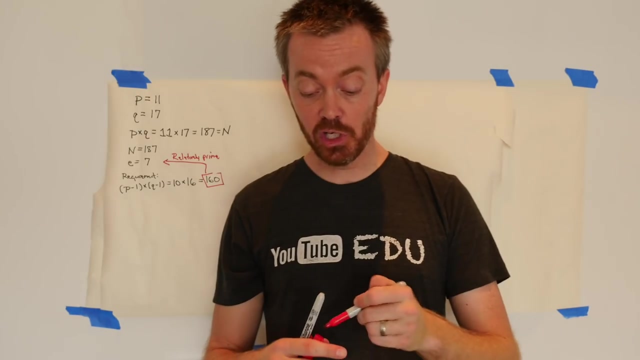 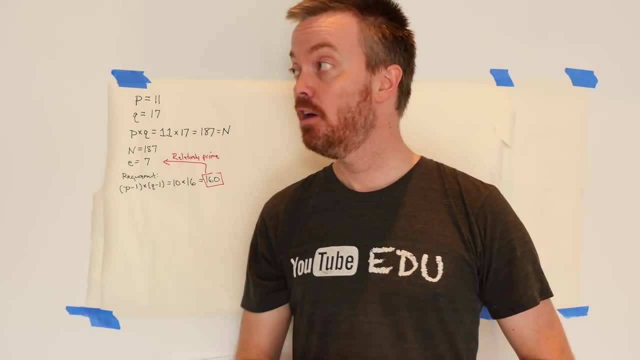 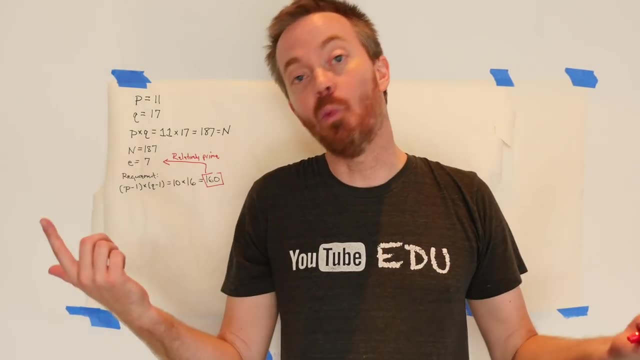 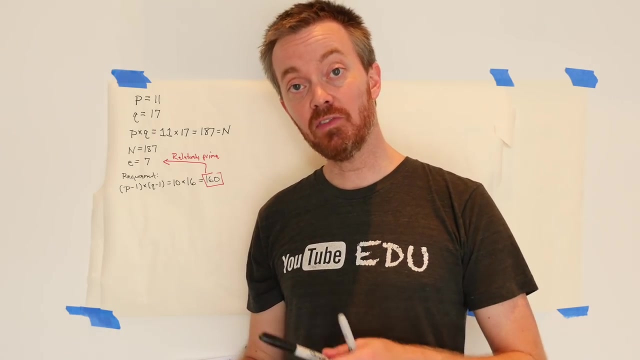 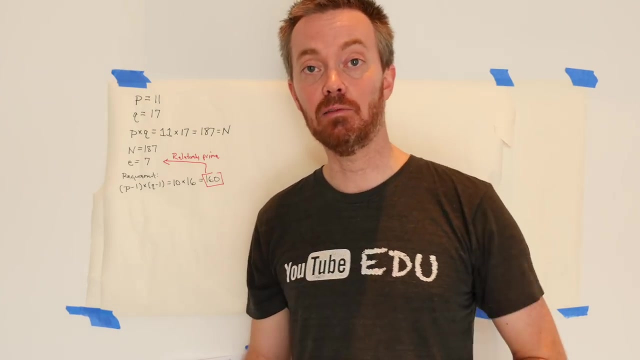 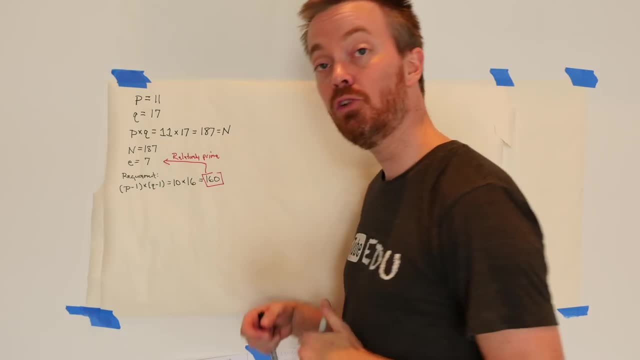 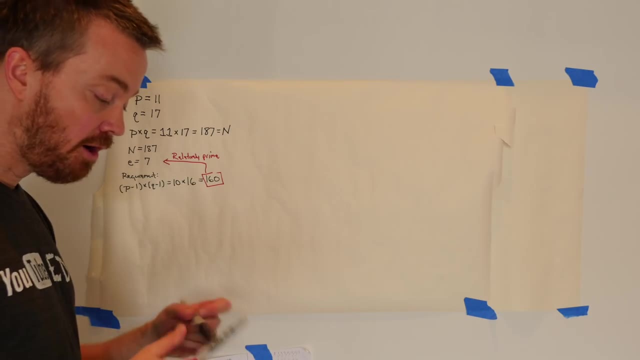 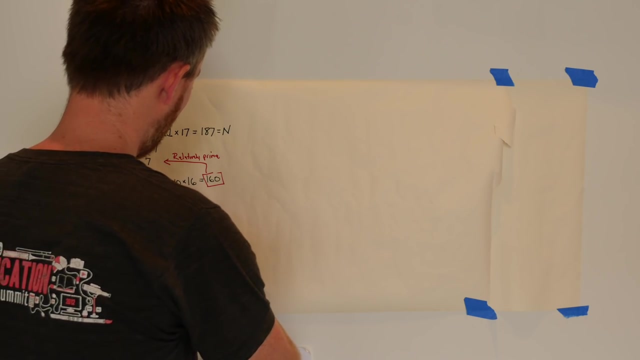 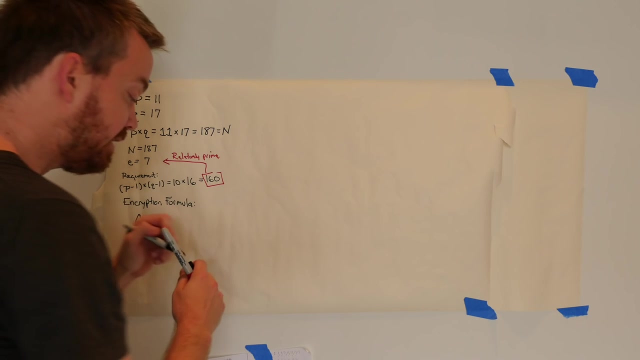 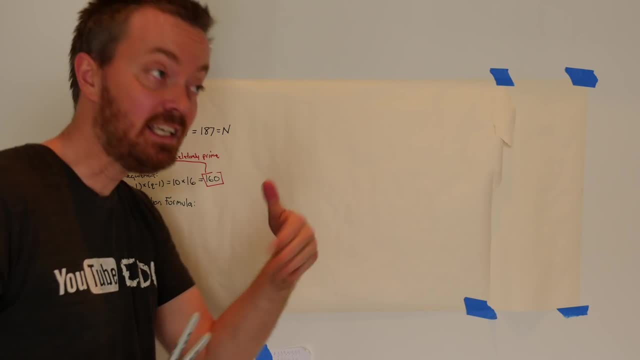 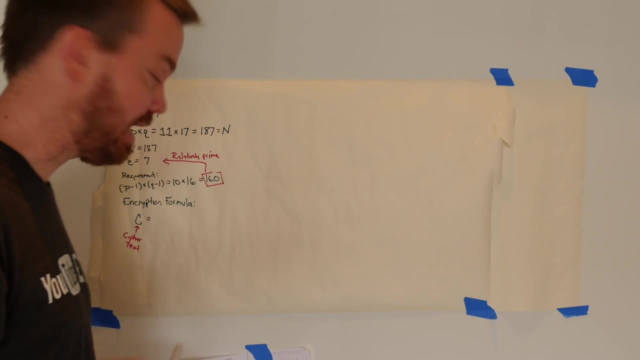 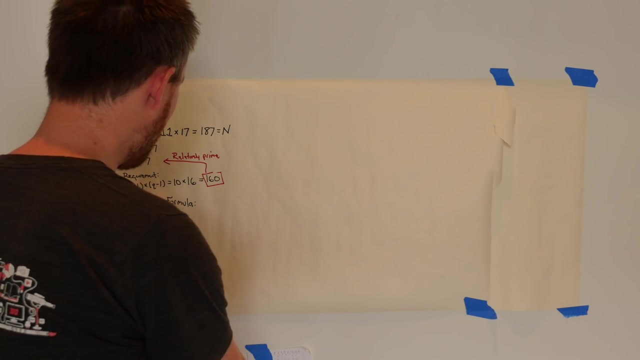 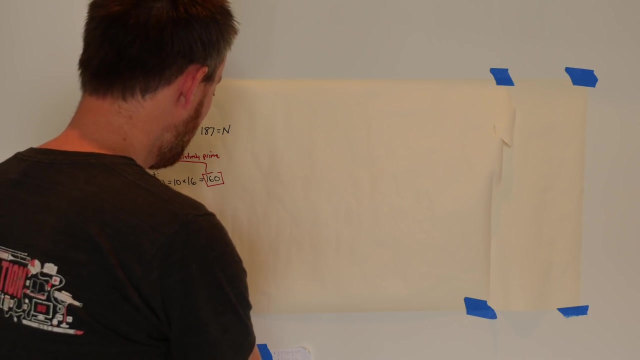 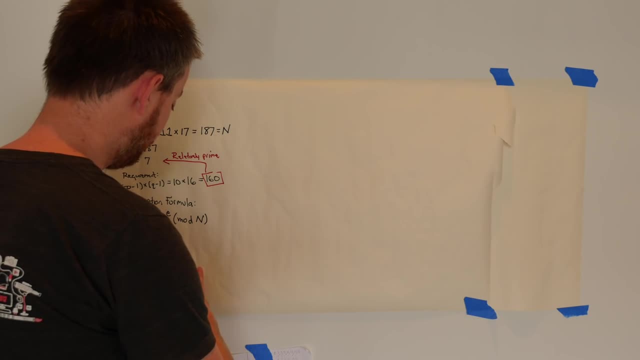 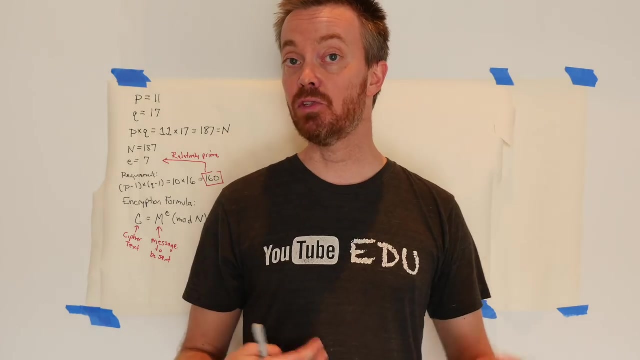 So m is going to be the message that we want to send. So the message to be sent Now, of course, since we're using computers, everything gets turned into binary zeros and ones, but that actually gets converted into something known as decimal, and that decimal version is what 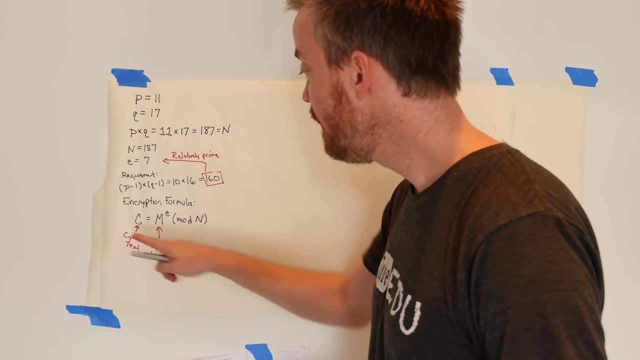 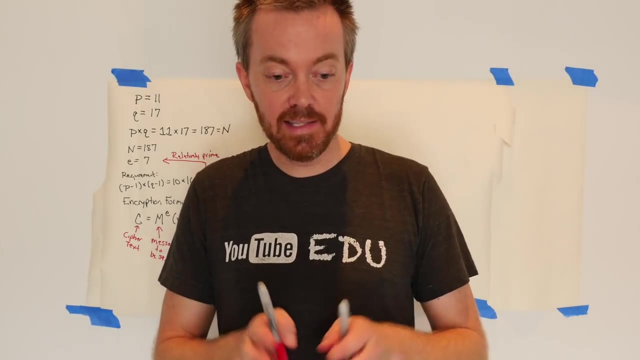 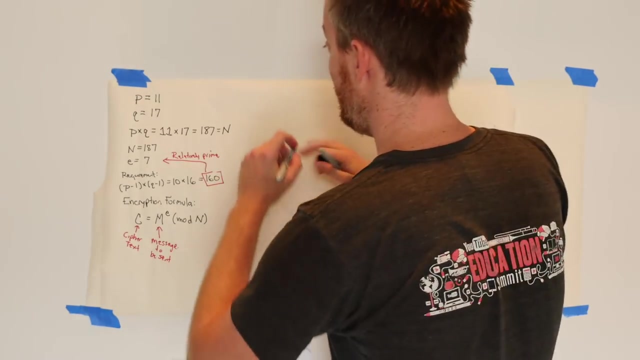 gets sent. We'll talk about that in a second as well. Let's talk about modular arithmetic. So modular arithmetic, it basically takes a number and it finds a number that's equivalent to it, and the number that's equivalent to it has to do with its remainder. So, for example, if I wanted to, 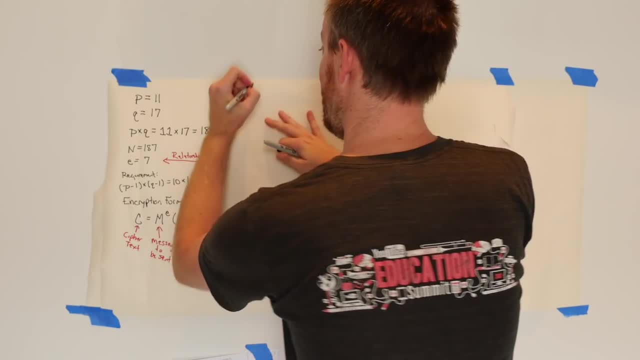 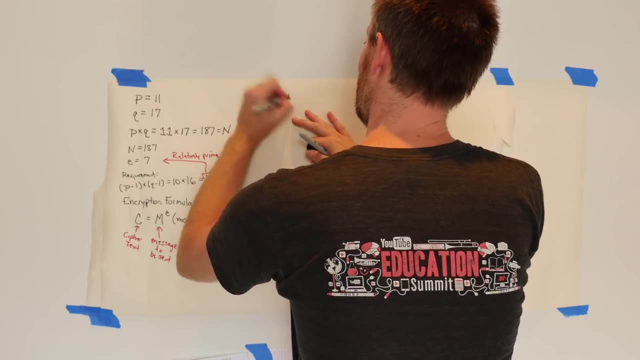 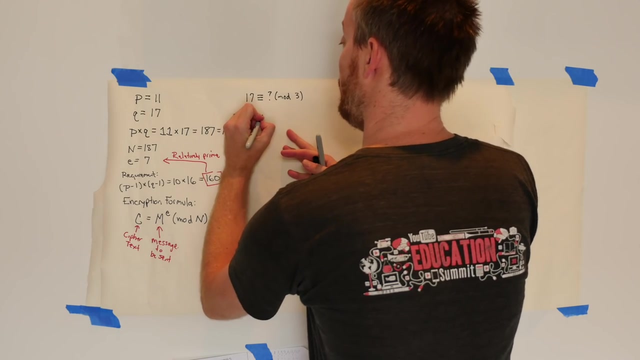 take, let's say, just a random example here. let's say 17 is equivalent to what we'll say mod 3.. So I want to know 17 is equivalent to what number- mod 3.. Well, what I can do is I can do long division. 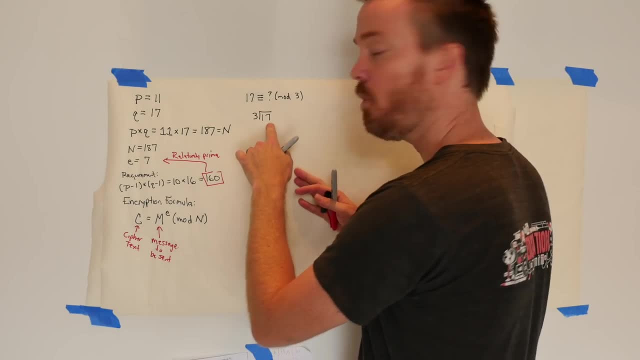 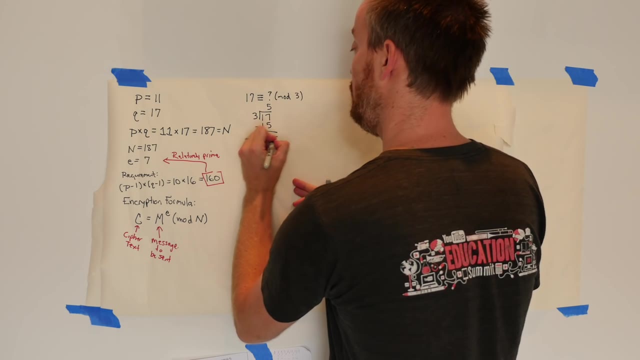 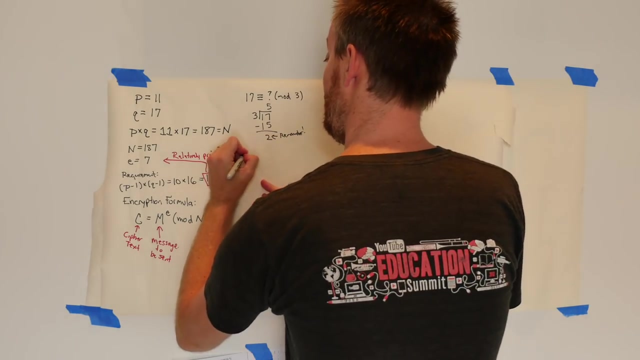 So 17 divided by 3. Well, 3 will go into 17. five times 5 multiplied by 3 is 15.. We subtract, we get 2. That's the remainder, That's what it is equivalent to. So we could say that 17. 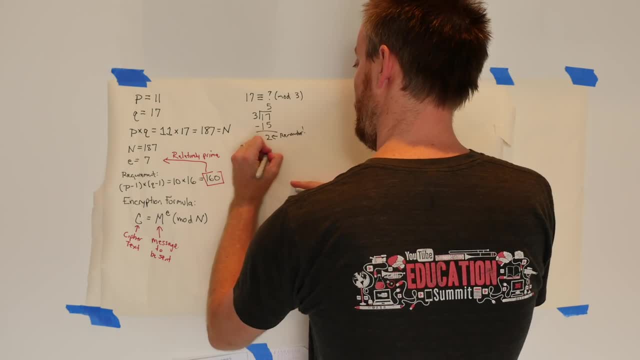 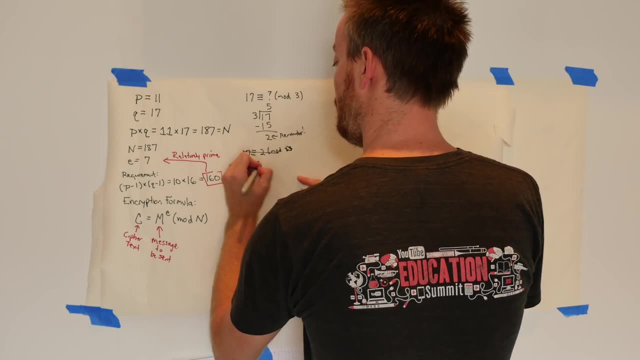 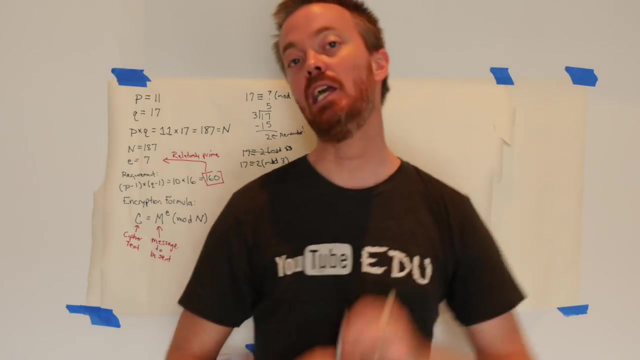 is equivalent to the number 2 mod 3.. So 17 is equivalent to 2 mod 3.. So you can see that mod 3 is equivalent to the number 3.. And we actually use modular arithmetic all the time, Every day. I bet you you use modular. 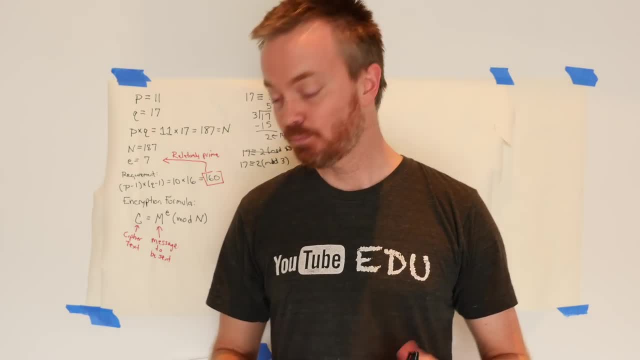 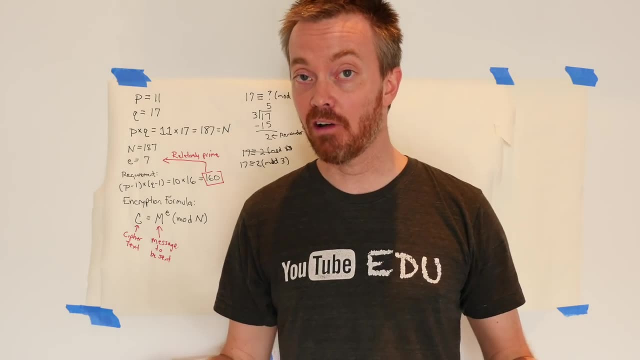 arithmetic. So if it's 10 am right now 10 am, and I say what time is it going to be five hours from now? Well, you don't say 10 plus five. You don't say it's going to be 15 o'clock, right You? 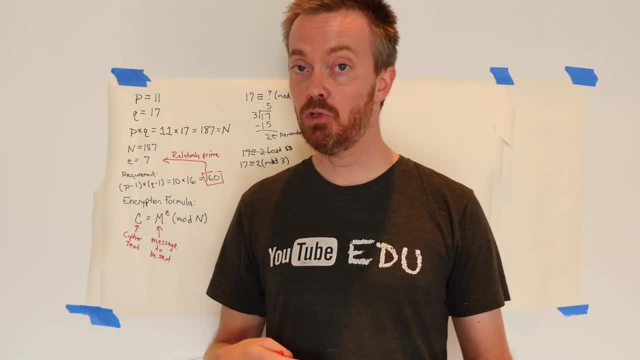 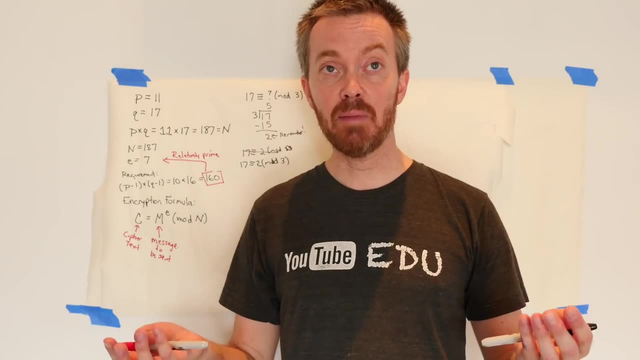 say it's going to be, oh, it's going to be 3 o'clock. What you're really doing when you do time is you're thinking about mod 12.. So 15, I'm really doing that- modulo 12.. Let's see. so 15 divided by 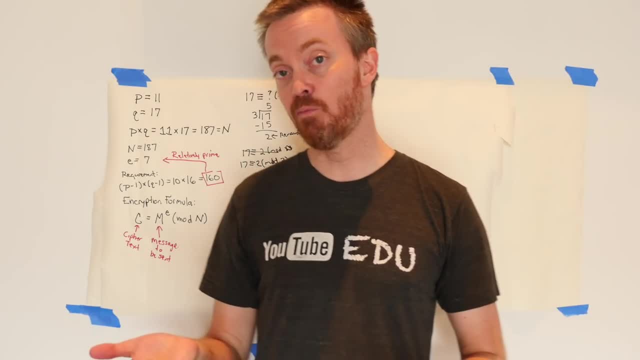 12 would leave a remainder of 12.. So we can say: 15 divided by 12 would leave a remainder of 12.. of three. So that's a common example of modular arithmetic that we do every day. You're basically just doing long division and you're thinking what's the? 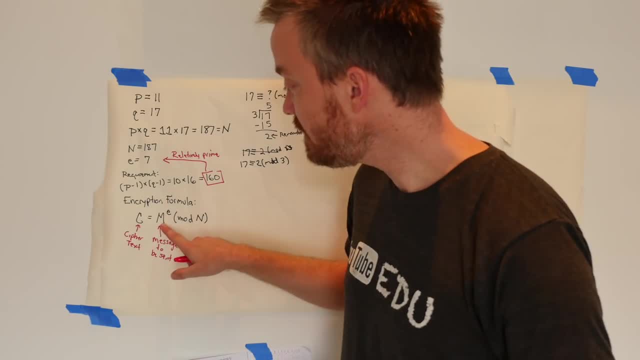 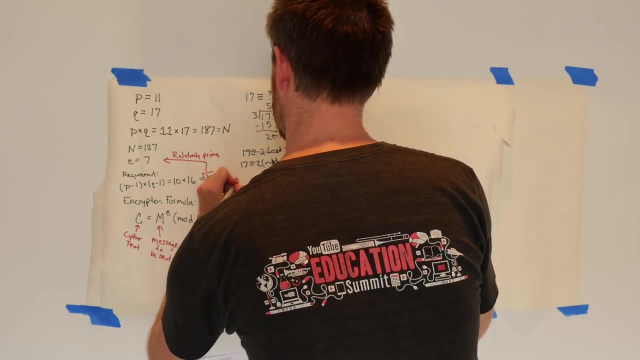 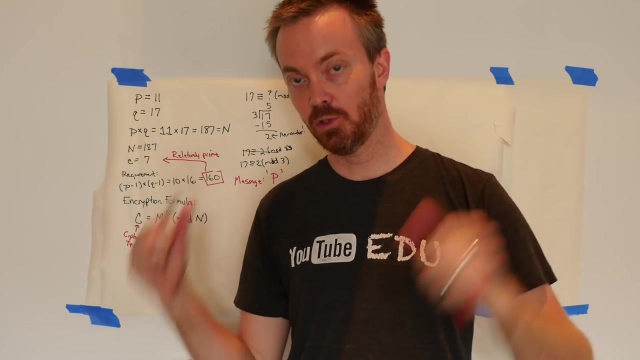 remainder. Okay, so M is going to be the message that we want to send. So suppose we just want to send a very simple message, Suppose the message I want to send, so suppose I just want to send the single letter P for yours truly. Well, you. 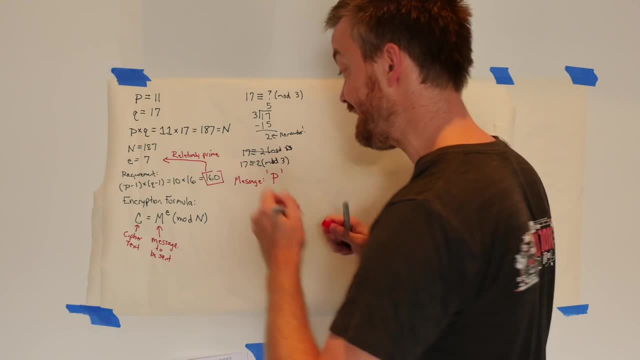 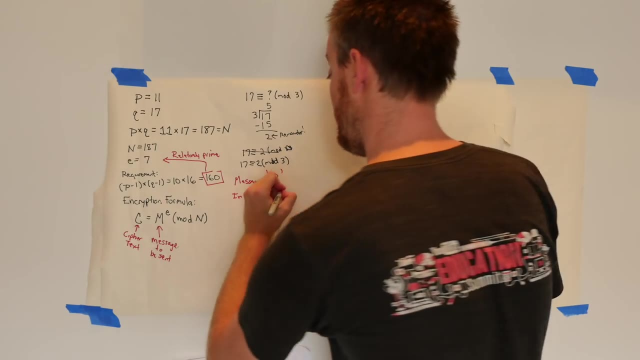 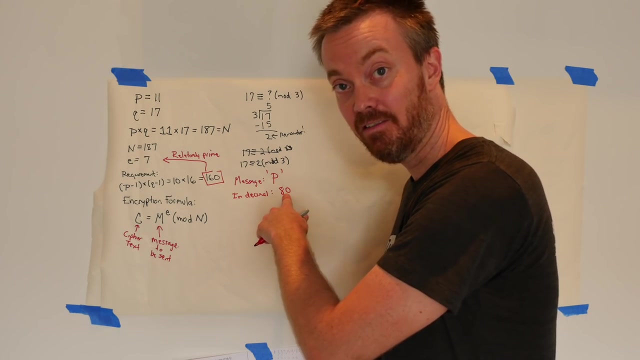 can look up this number in binary- I forget what it is, but in decimal. in decimal, the number P is represented by the number 80.. Okay, so that's what I'm going to send. I want to send this number 80 via the internet, So, okay, so. 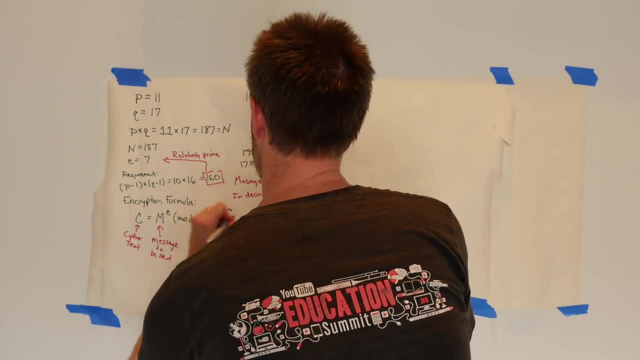 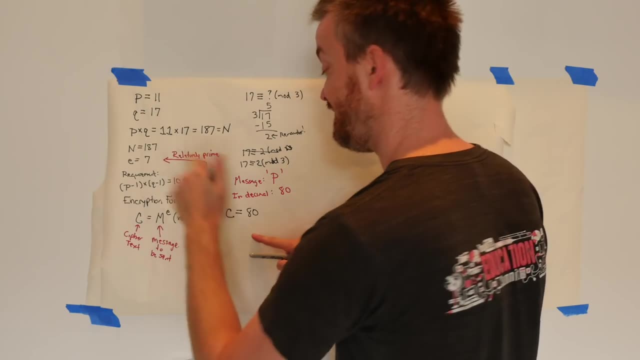 now I use my formula here. So C is going to be equal to the message, which is the number 80. I raise that to the power of E, which is 7. So 80 to the 7th, that's a pretty big number. And then I have to do that. 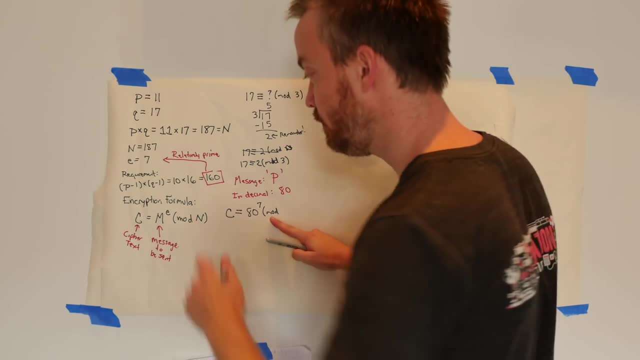 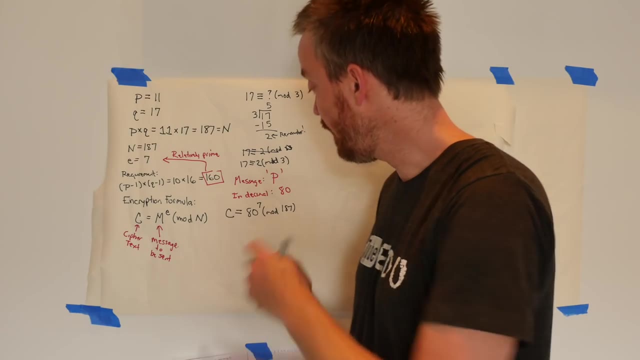 modulo. so mod or modulo the number N, and my number N here is 187.. So there are ways to do this. you know a computer can do this. I actually put this either- I think I put this in Google or Wolfram Alpha. you can use that one as well. 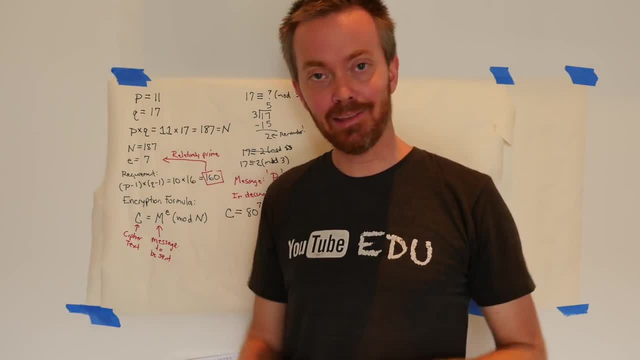 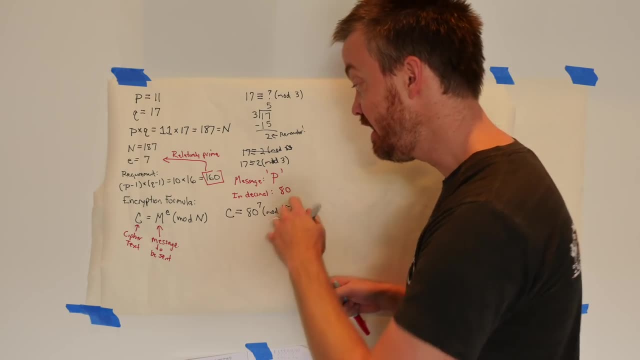 There's a way to do it, to do it a little bit shorter by hand. I'm not going to talk about that. but if you take 80 and raise it to the seventh power and then you were to do long division with 187, it turns out that that number 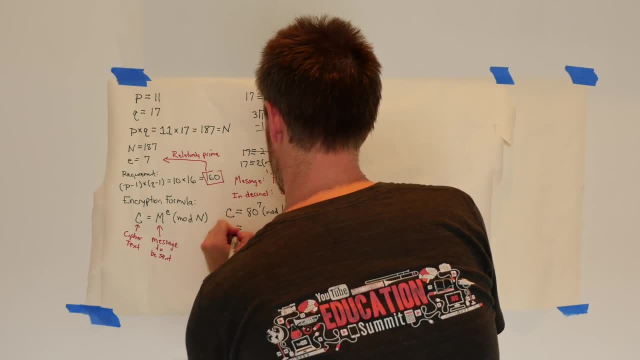 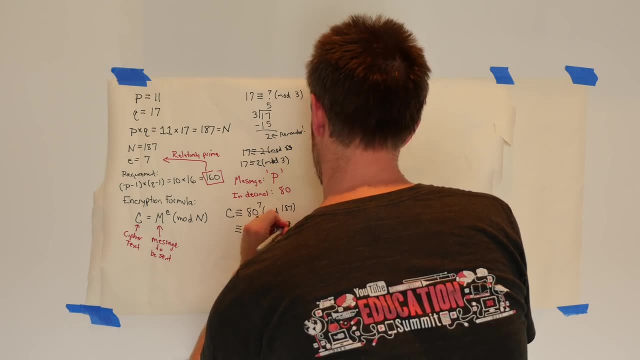 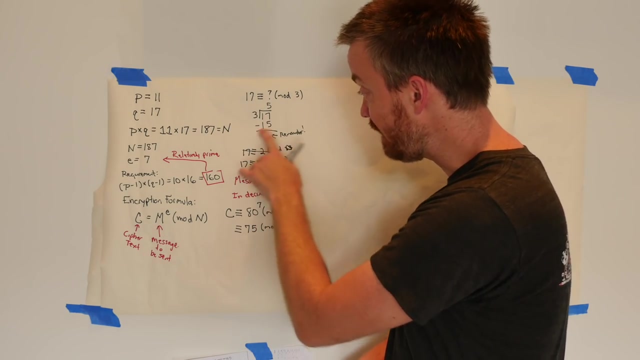 is going to be equal to. it's going to be equivalent to the number 75 mod 187.. So if I take 80 to the seventh, divide it by 187, do all the long division, I'm going to find that my remainder, when I'm done, is going to be 75.. That is going to be. 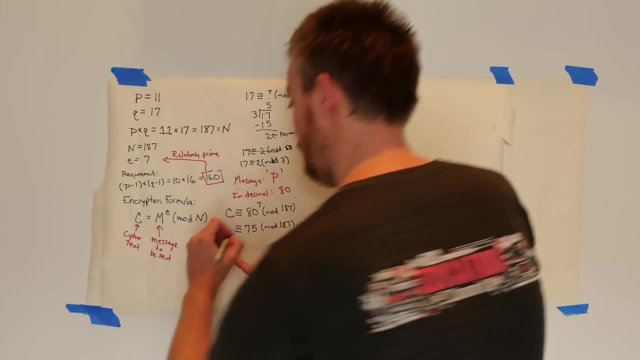 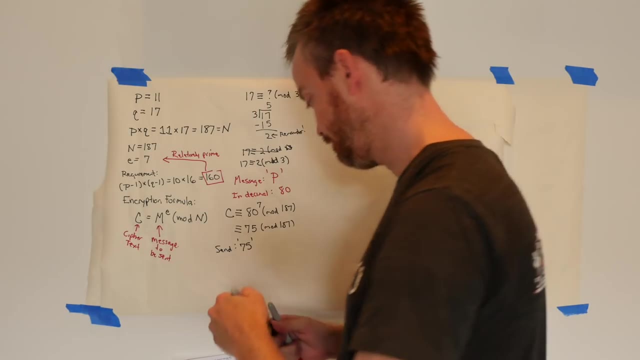 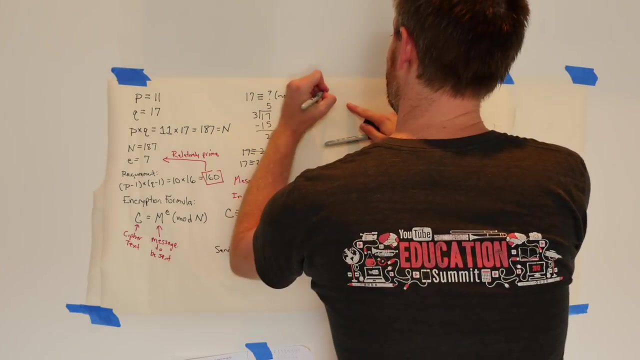 the ciphertext. So that's what gets sent. So we send. we send this number 75 on the internet. Okay, so what happens now? So what we do now is we calculate something new. We have to calculate. we take our number E. 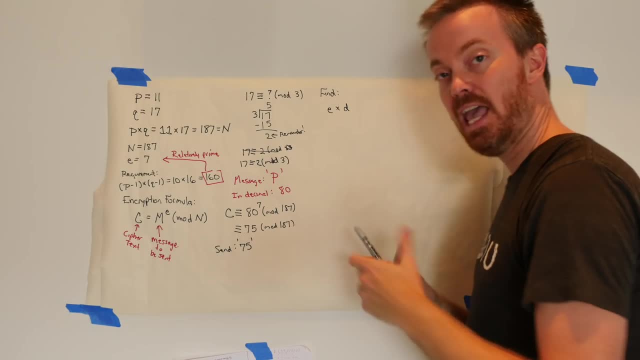 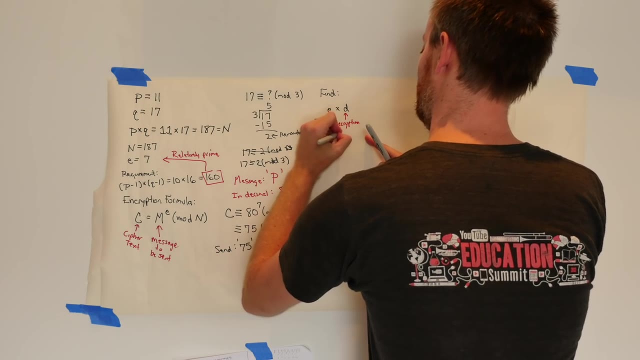 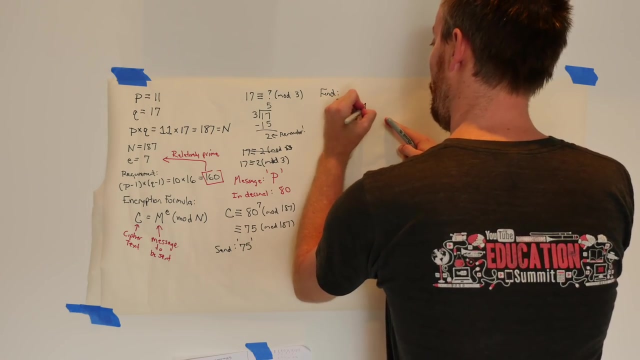 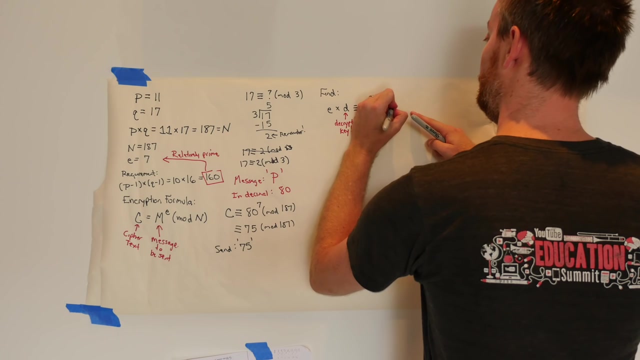 and we multiply that by some number D and this number D is going to be the decryption key. So this is going to be our decryption key And we want E multiplied by D to be equivalent to the number 1.. When we do mod, we take p minus 1 times q minus 1.. 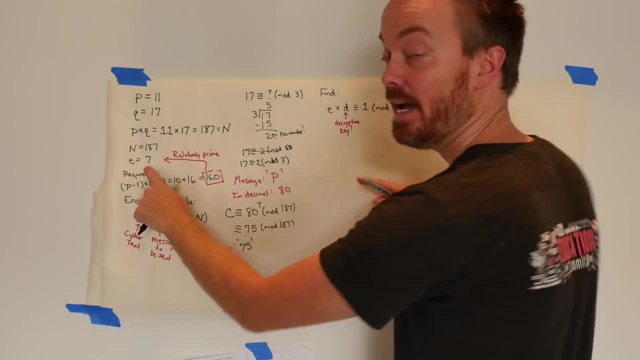 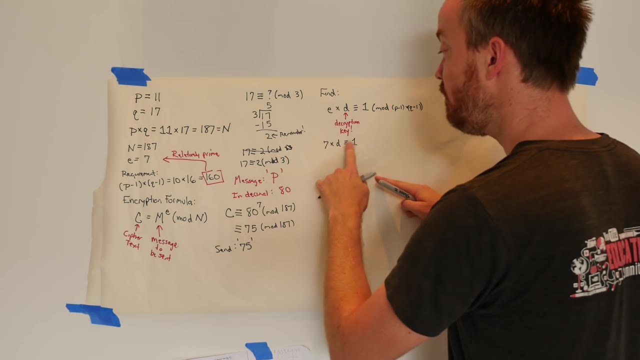 Okay, so we said that the number E we already picked, that that's the number 7.. So I have to take 7 and multiply that by D and have that be equivalent to the number 1 modulo. well, p minus 1 times q minus 1.. 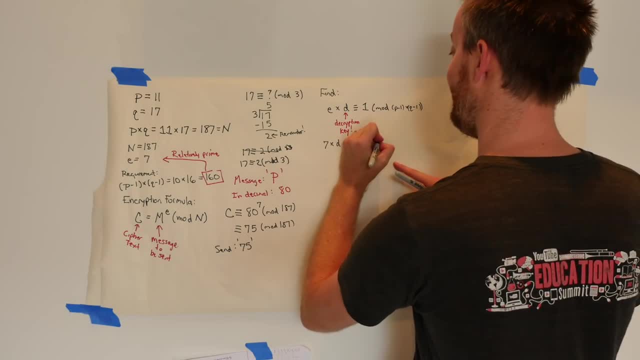 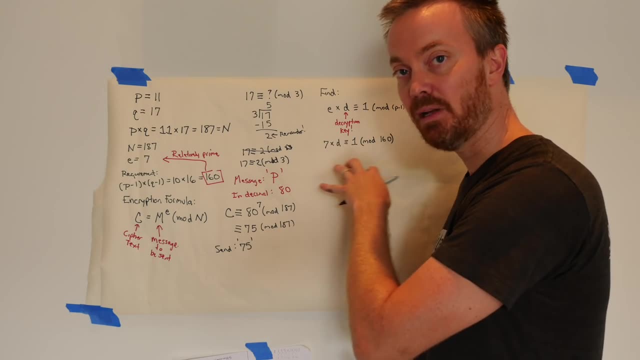 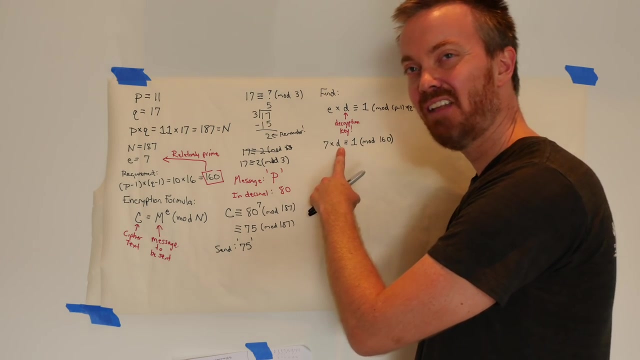 We just computed that over here. That was the number 160.. And the reason why you want these numbers to be relatively prime. otherwise some funky stuff can happen at this step. That's the reason why this needs to be relatively prime. So I have to take 7 multiplied by what number? I've got to do long division. I've. 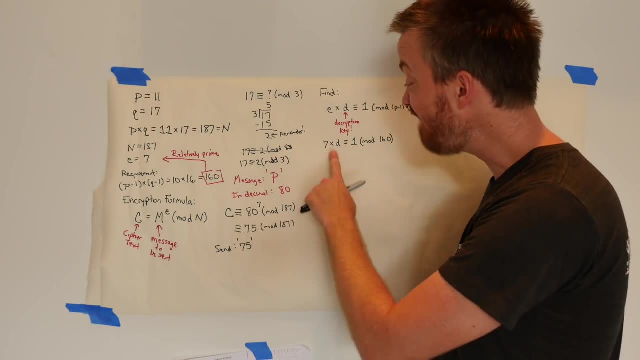 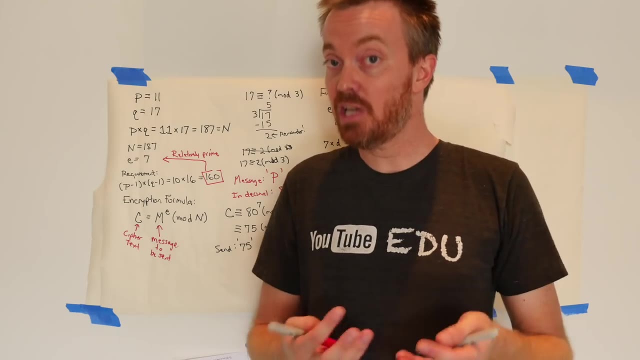 got to divide, in this case, by 160, and I have to get a remainder of 1.. I have to figure out this number D Now you think. well, I don't know how to do this. It turns out there's something called the Euclidean Algorithm that actually 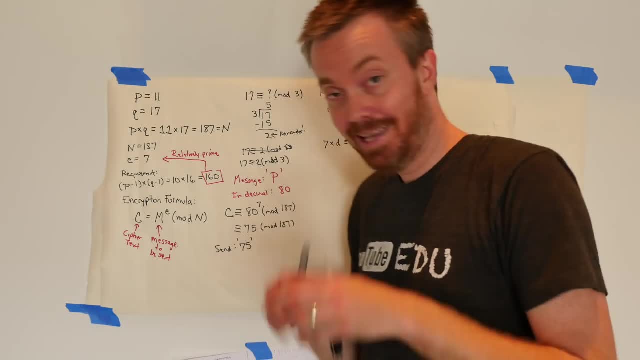 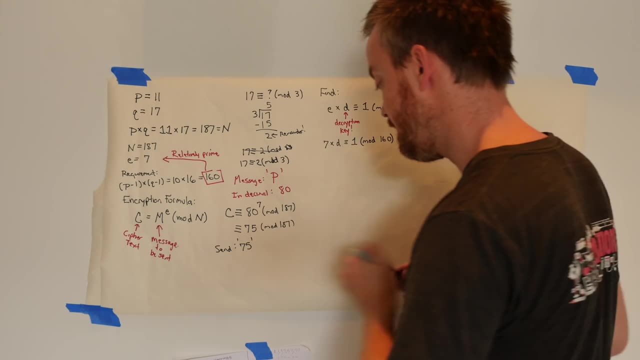 enables you to find this relatively quickly. So again, I'm going to leave those steps out. If you're interested, let me know, We can talk about it. So it turns out that, to get this number D, it turns out that this number D is equal to the. 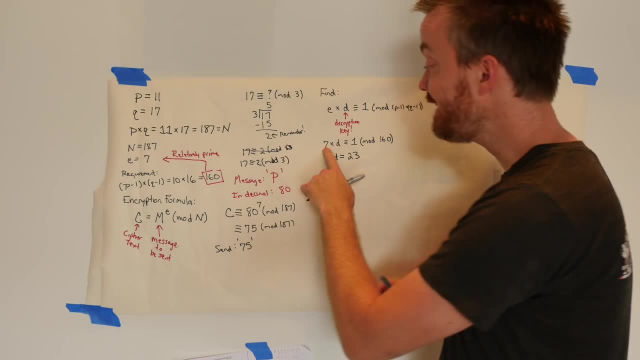 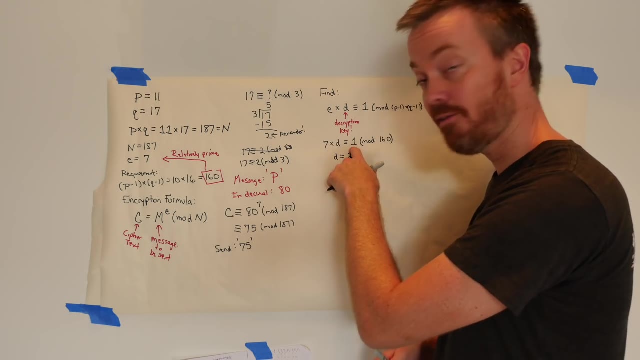 number 23.. So if you take 7 and multiply it by the number 23,, you'll get a new number. Divide that by the number 160, you're going to find out that you have a remainder of 1 at the end. Okay, and this is the decryption key. This is important. 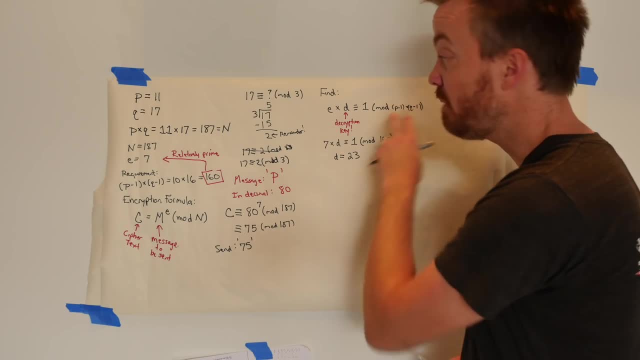 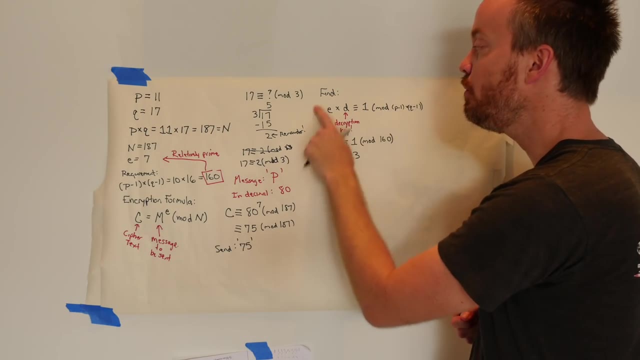 And the only reason why you're able to figure out this number is because you've kept P and Q private. Nobody knows those numbers, So to work out this step is super, super difficult. The only way to solve it we know right now is to use 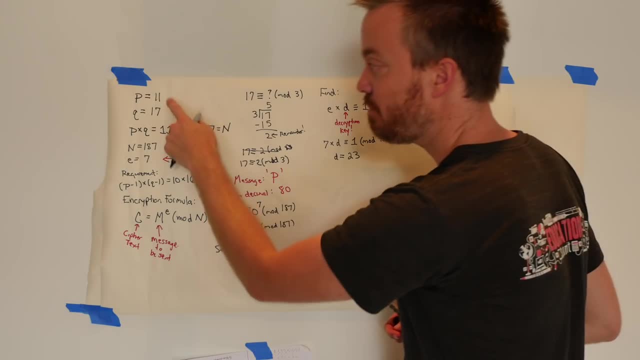 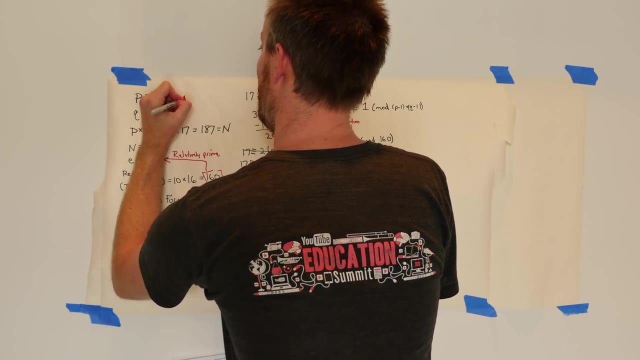 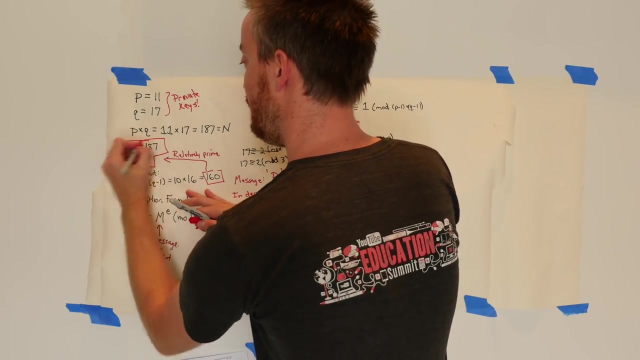 brute force. So the only way to get this decryption number D is by already knowing these two numbers, P and Q. And again, these are your private keys. Your private keys. So the numbers 187 and 7, the numbers N and E, those are your public key. So anybody. 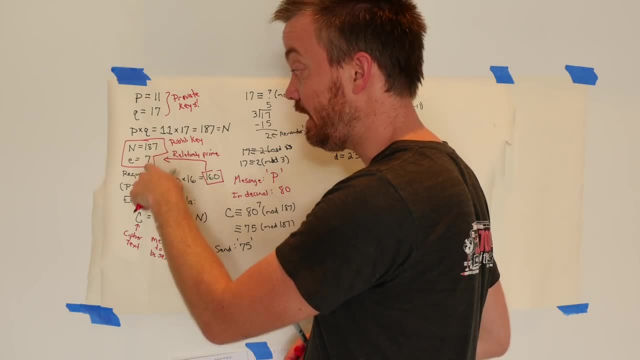 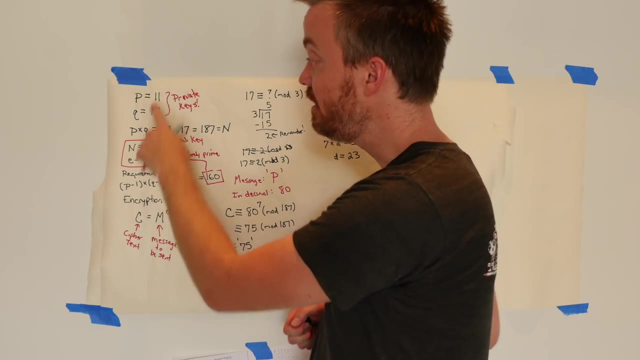 again think about like a telephone directory. Anybody can look up the public key, these two numbers. They see 187. Again, intuitively, the idea is that these are going to be really large in practice, so that people don't know what P and Q. 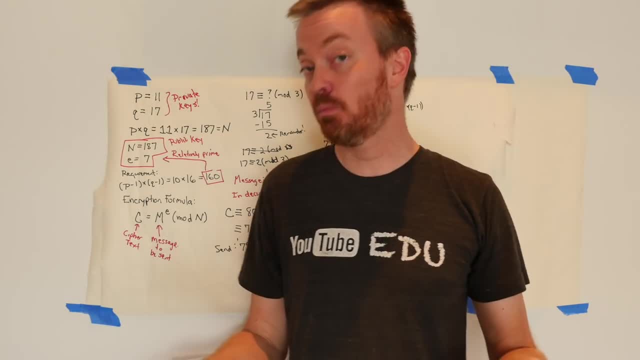 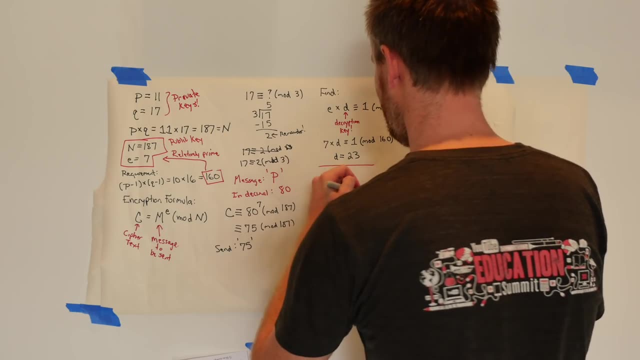 are, Those are your private keys, And this is where we get the terminology public and private key. So okay, we get this number. D equals 23.. So now to decrypt. so now to decrypt the message. to decrypt, we use the following: 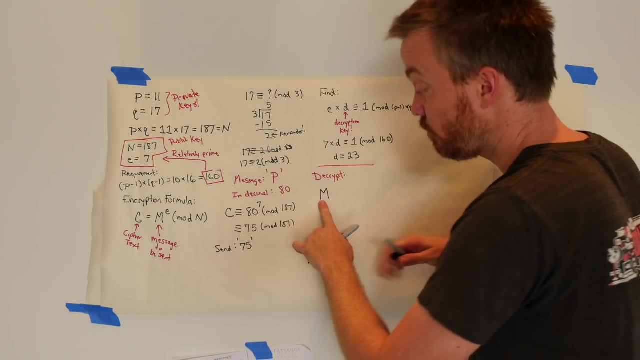 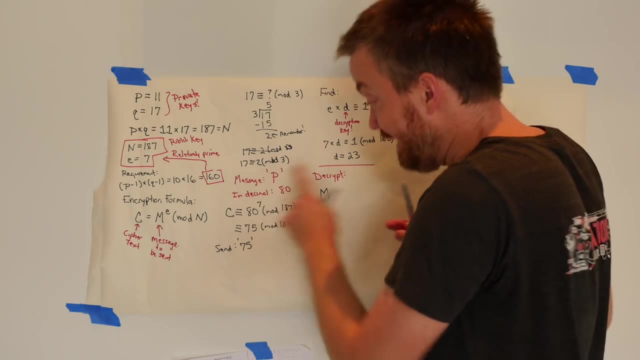 formula: We want to get the original number. the original number M, which was the original message, So M is going to be the message to be sent. We sent the letter P So M to get the original message sent. we're going to take the. 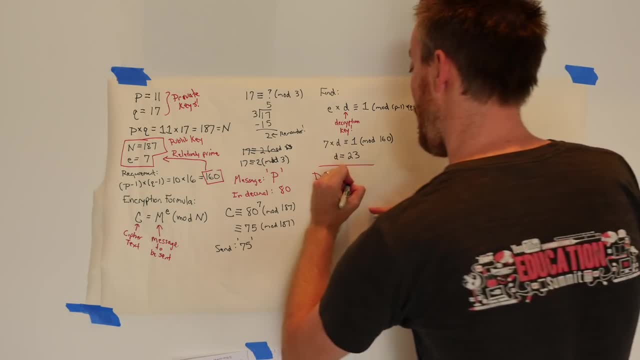 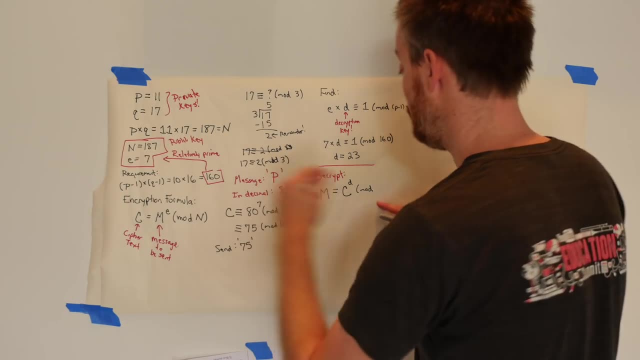 ciphertext C. we're going to raise that to the power of D And again we take it, and this can be done with even lower blocks, and this is coupled with a case. we do mod the original value of m, which is 187.. Okay, so I'm trying to. 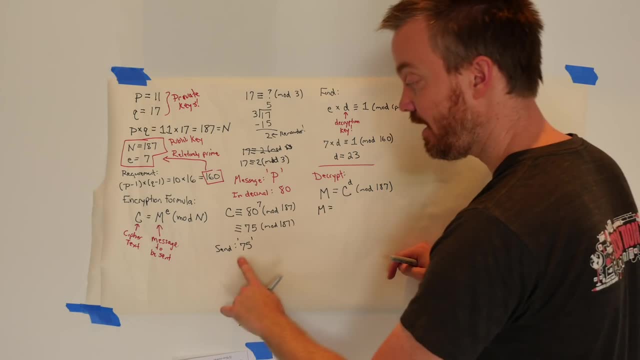 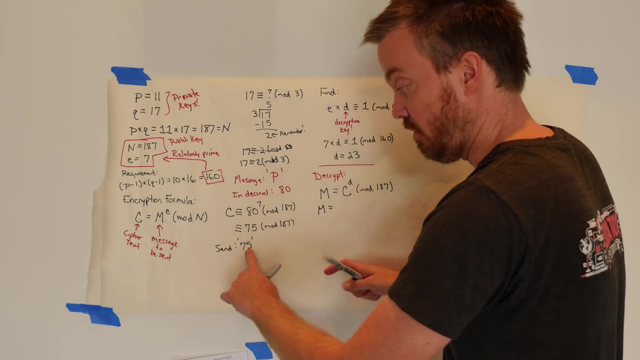 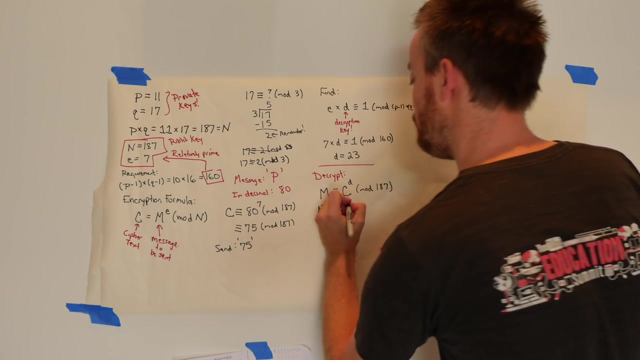 recover this original number m? C was the ciphertext, That's what we received, this number 75.. And again, maybe somebody intercepted it and they saw that the number 75 was sent, But without knowing this value of d, you're in big trouble. So 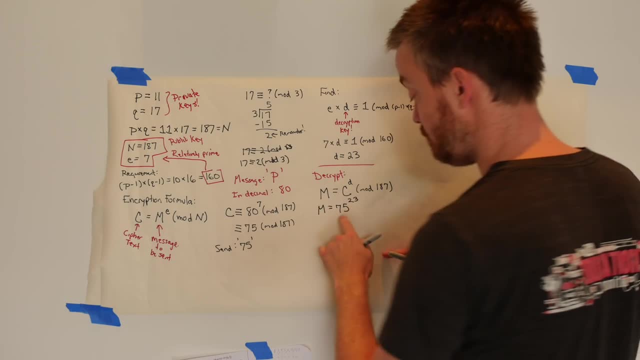 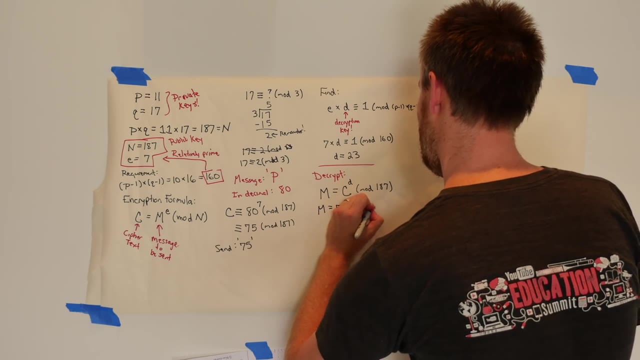 75 raised to the power of 20,, excuse me, 75 raised to the power of 20,. 75 raised to the power of 23, mod 187.. Again, you know you wouldn't want to do this by hand. 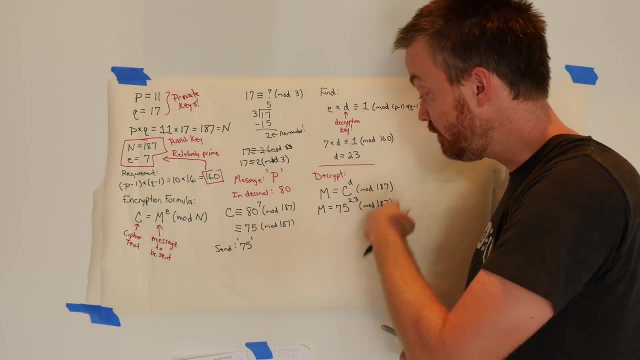 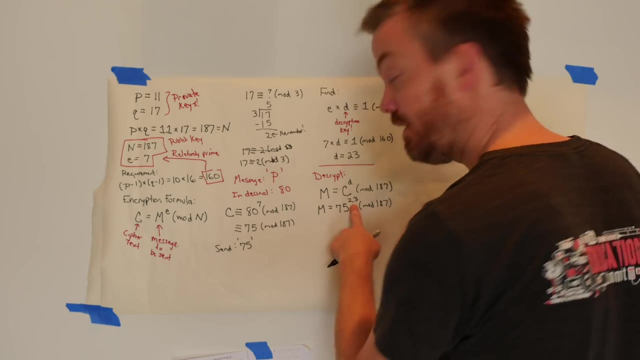 There are ways to break it down and do it by a calculator. Again, I think I put this into Wolfram. So if you compute this, m equal to 75 raised to the power of 23 mod 187, you get lo and behold. 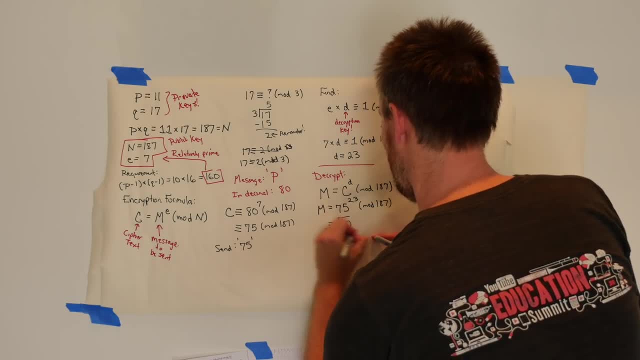 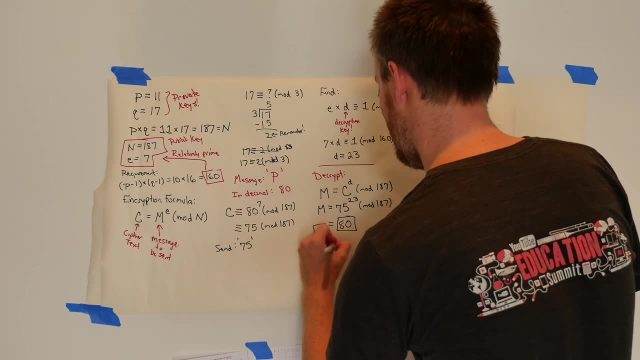 m equal to 75, raised to the power of 23 mod 187.. You get, lo and behold, you get the number 80.. Ta-da, And the number 80 was the original number that we sent. And again, the number 80 now corresponds to the letter p, So that's. 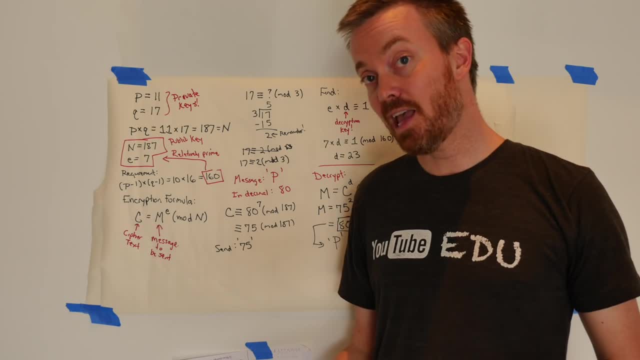 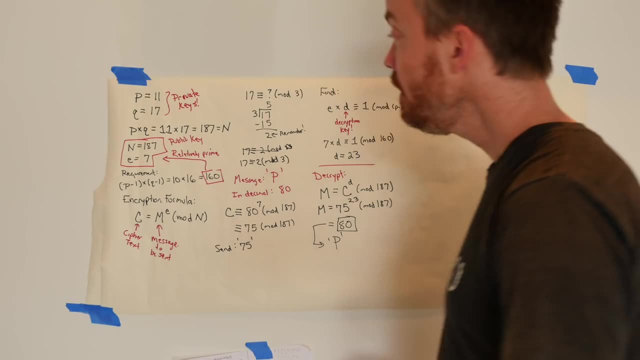 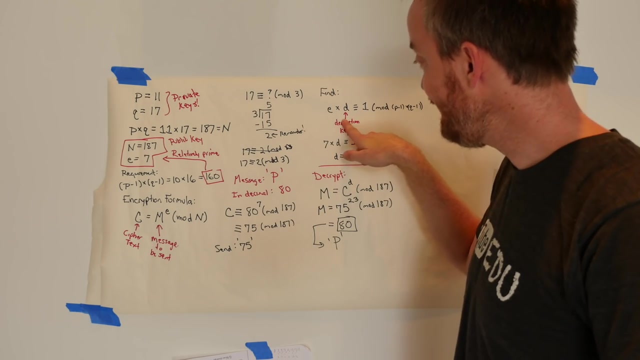 how this encryption method works, And this is known as RSA encryption, after it's the first initials of the last names of the people that came up with it. So that's the basic idea. And again, it's super difficult to find this number d, this decryption key, without knowing p and q. And again, that's. 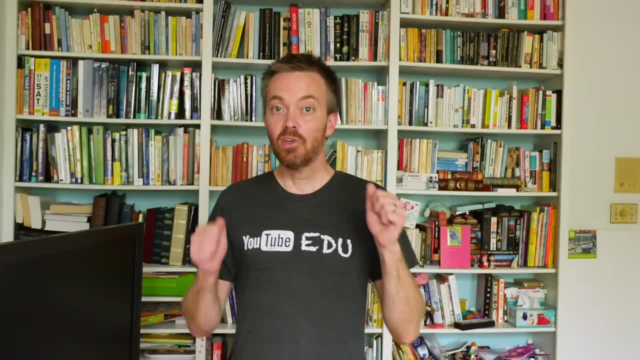 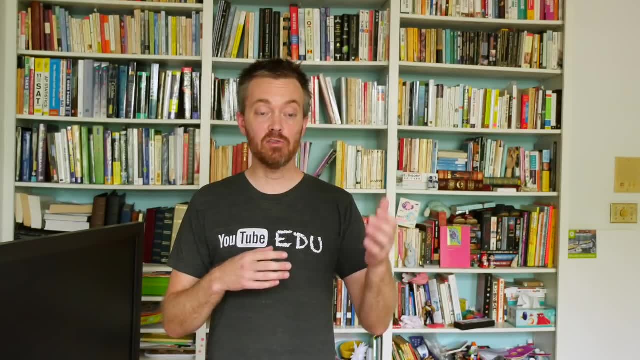 the brilliance and that's the magic. So in our example again, we picked small values for p and q to make the math manageable. In actual practice, the values for p and q, and therefore the resulting value for n, can be ginormous. So for 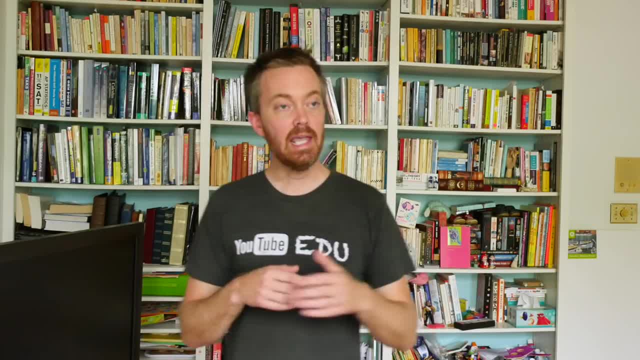 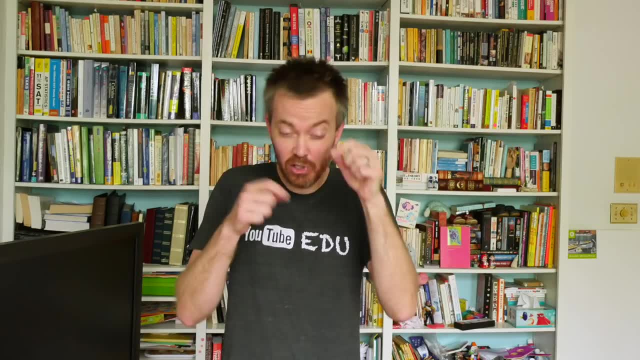 example, in really important banking transactions n can be larger than 10 raised to the 300 power And 10 raised to the power of 300, you know you write that down: 10 raised to the 300, it looks kind of innocuous. It's hard to feel. get a feel for how big of a number. 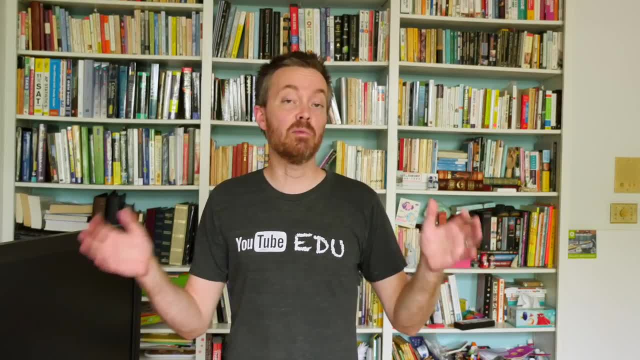 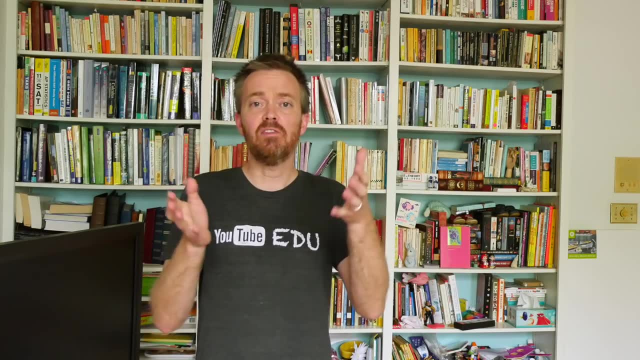 that is, But that's easily. that number is easily larger than the number of atoms in the universe. It's a by far, it's a gargantuan number And I was reading that if you take even you know a hundred million personal computers all working. 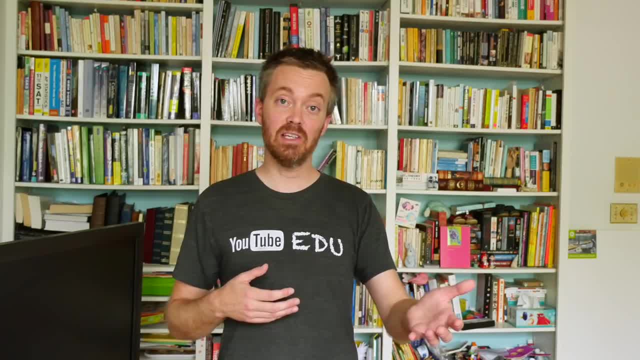 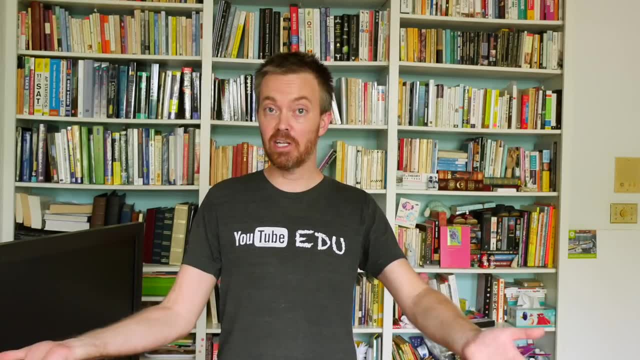 together, it would still take over a thousand years to crack one of these codes. So, again, from a brute force perspective, it's simply: these codes are perfect for our everyday use and function, which I think is really cool. So you know again, this is this issue of. 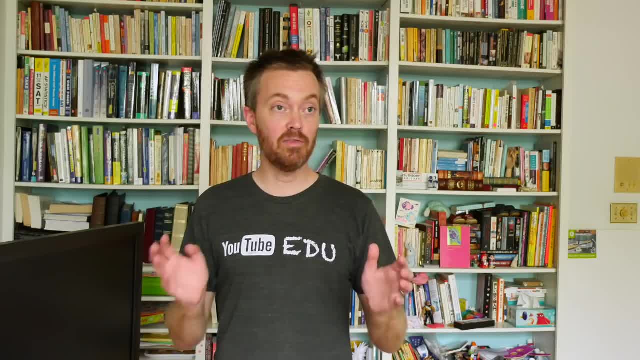 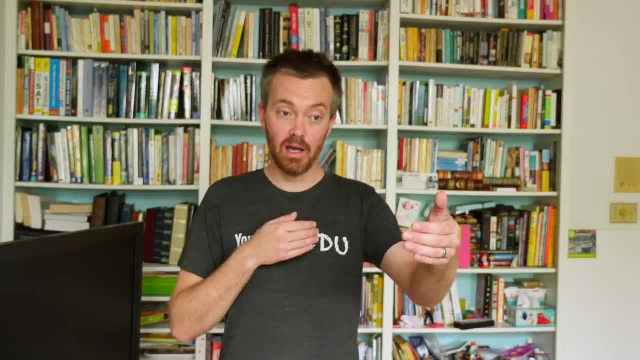 key distribution had been central to cryptography forever. It's hard to sort of overstate the importance of it. It was one of the central concerns of having a good, a good system And these people through some. you know I'm gonna say relatively simple. you know it deals with prime numbers and 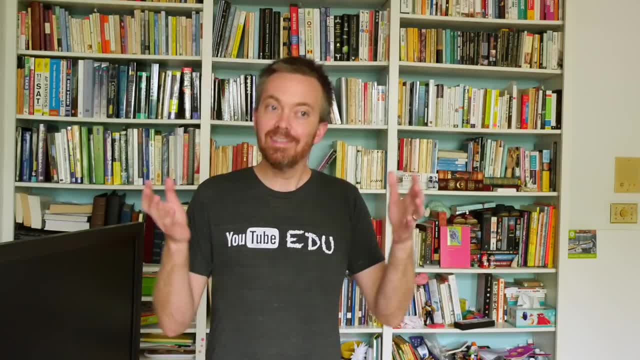 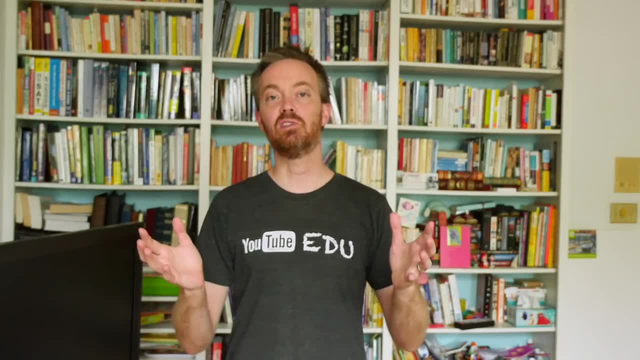 factoring and modular arithmetic with some relatively simple mathematics. but the way that it was all put together was just absolutely brilliant. I mean just brilliant, the mark of genius, the way that they did this. So I think it's great And again, you know, it's things that we take for granted, but the way that 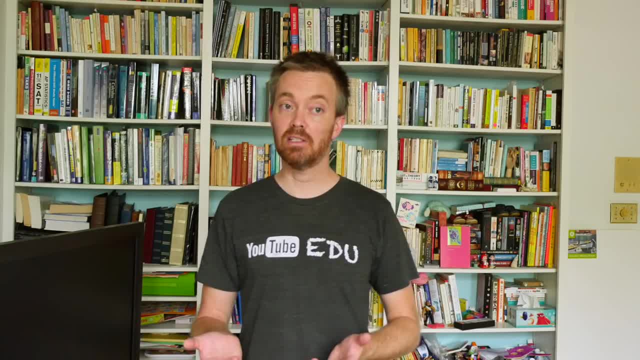 we use the internet now. it wouldn't be possible without some of this mathematics, And I think that is really cool And that's part of the reason why I love math, because you know there's all these things going on behind the scene that we 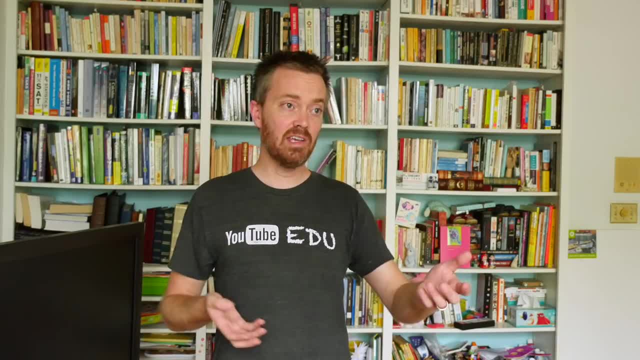 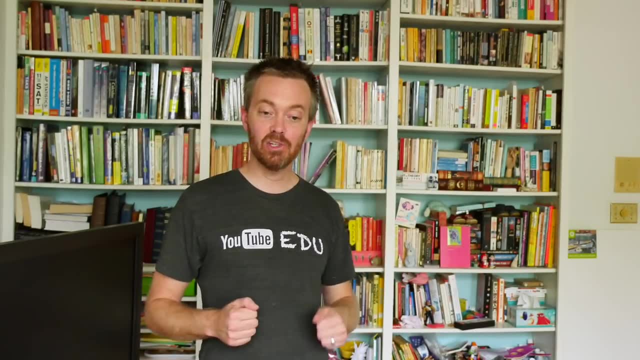 all a lot of times don't really see or think about that- make a lot of things that we use on a day-to-day basis useful and possible. That's why I love math. I think it's great. So once again, a big shout out to. 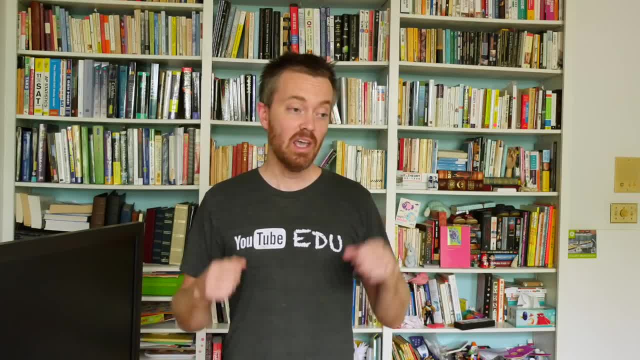 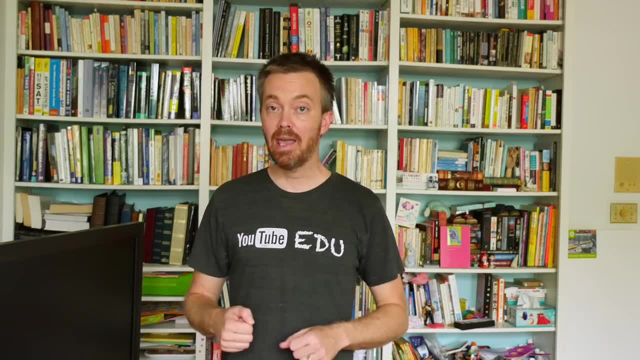 the making and science team at Google. They made this video possible. If you like this video, please thumbs up it, share it- you know- Facebook, Twitter- with the hashtag science goals- and stay tuned. I love making these types of videos and 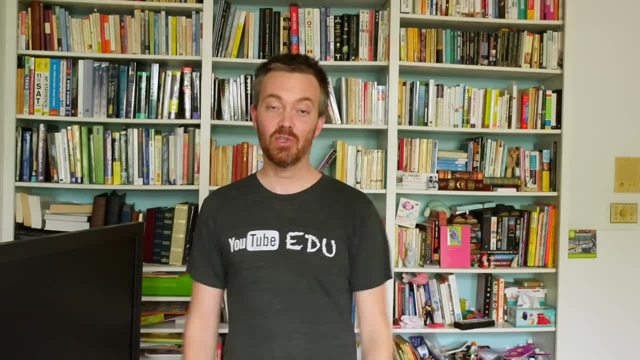 I like my technical ones as well, but these are fun too, So stay tuned for more of these, as I'm going to keep making them. Thanks,